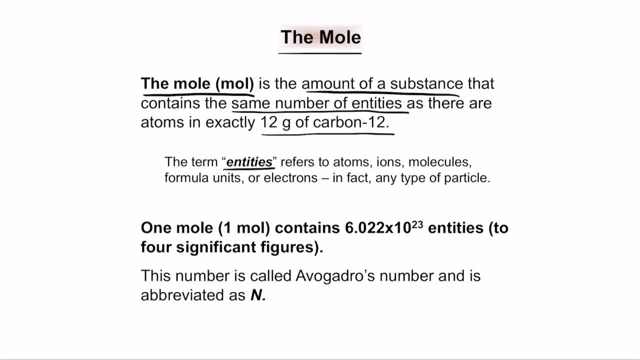 how many entities are there? So the term entities can refer to atoms, ions or molecules. can also be formula units. If you have an, if you have an ionic compound, it can be electrons. If you have a single atom and can be a metal and in fact it can be any type of particle. 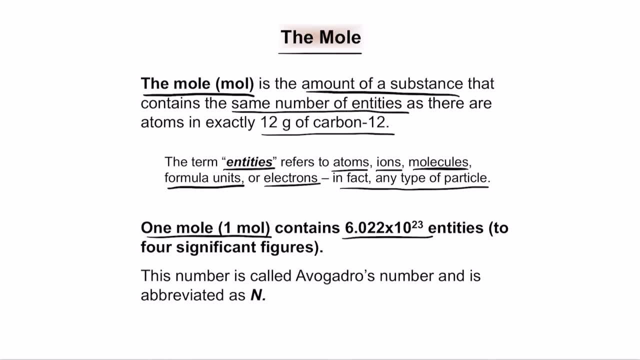 So one mole contains about 6.022 times 10 to the power 23 entities. So if you have a single atom it can be any type of particle. So one mole contains about 6.022 times 10 to the power 23 entities. So this is the number of particles in a single mole of a. 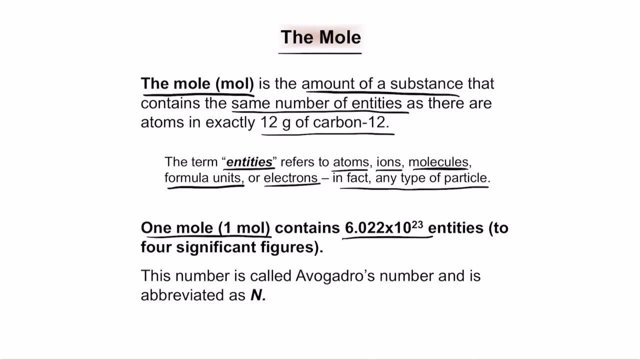 substance. So this is given to four significant figures. So this number here that you get here is called the Avogadro number and is abbreviated by the symbol n right. So whenever you see n here, so n refers to 6.022 times 10, to the power 23 per mole. So this is the 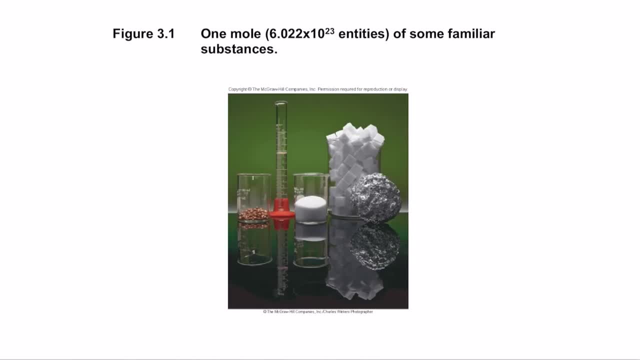 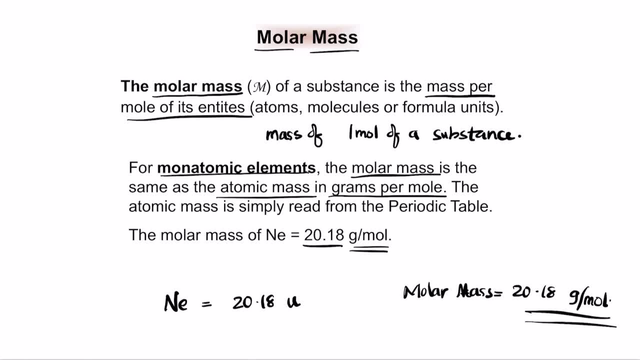 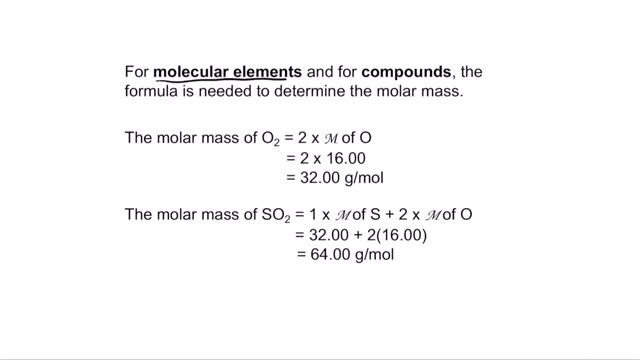 same. the unit is what differs in the value, so it can be simply read from the periodic table directly as well. so even the molar mass can be read directly from the periodic table if you have molecular elements and for compounds the formula needed to determine the molar mass is similar to: 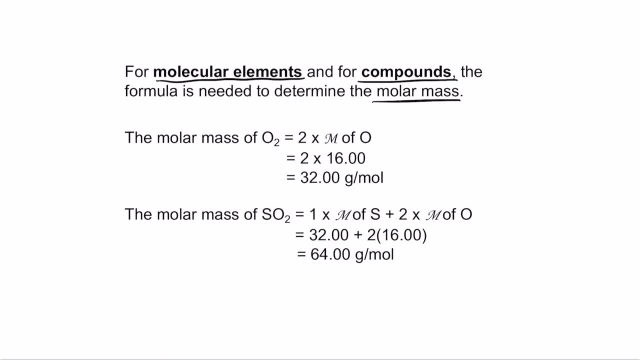 that of the molecular mass, so molar mass. here again we calculate two times the molar mass of each individual element. for example, if you take oxygen, we are taking twice the amount of individual quantity of oxygen, so that's 2 times 16, and we change the units to gram per mole in the same way. 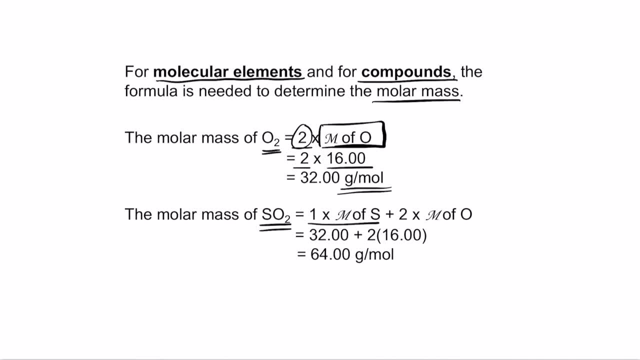 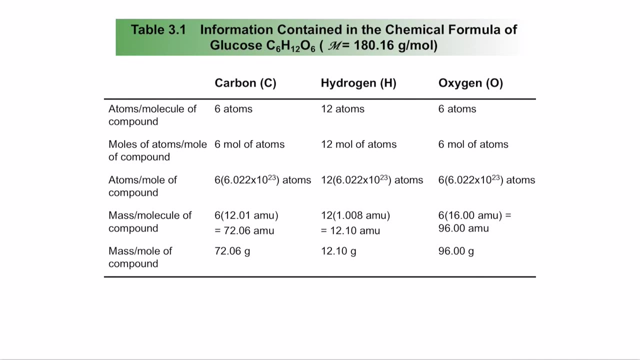 so to we write one times the molar mass of sulfur into two times plus two times the molar mass of oxygen and that gives you 32 plus 32 that's 64 gram per mole. so remember the units, really important. gram per mole. now. so when you take the exact quantities of a substance, if you take glucose, 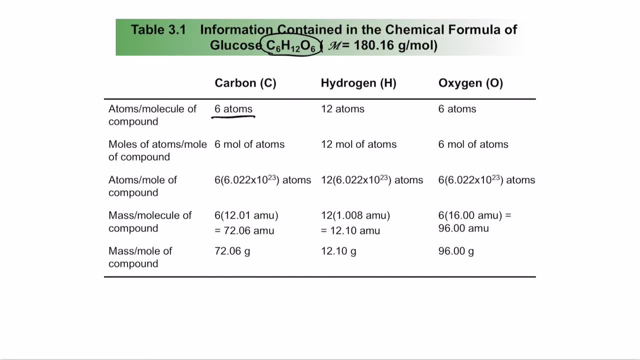 in glucose, you have six atoms: six carbon atoms, 12 hydrogen atoms and six oxygen atoms. in terms of the moles of substance, there are six moles of atoms of carbon, there is 12 moles of hydrogen and there's six moles of oxygen. and when you want to calculate the exact number of atoms, 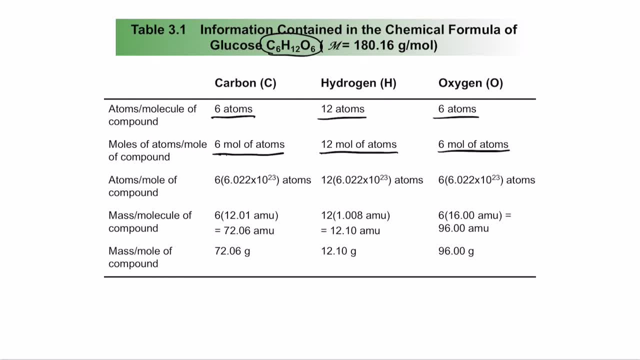 inside them, then we can calculate it by multiplying the mole with the avogadro number. so multiply the mole with avogadro number. that's when you get the total number of atoms. when you want to calculate the mass of the molecule, of the compound, of the compound, we can calculate it with the atomic mass unit. but 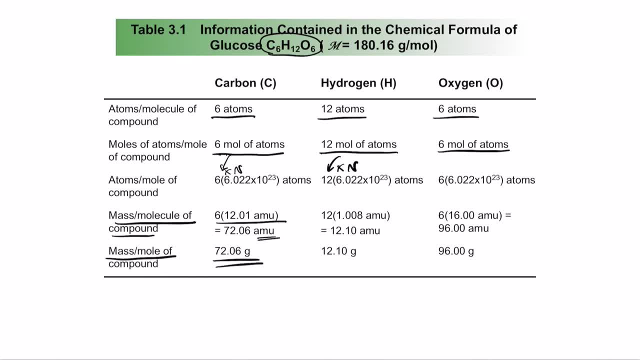 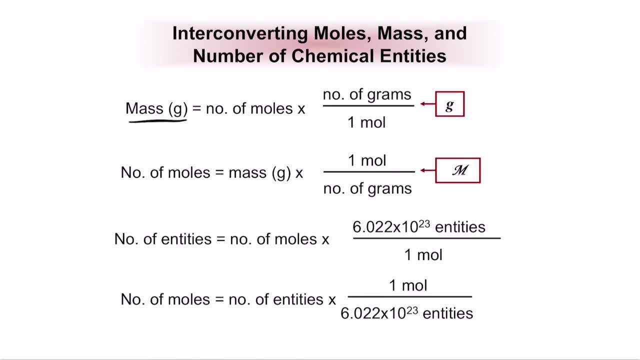 mass per mole can be calculated as grams. So that is the only difference between the other quantities and here. So now, when you want to calculate the mass, you can multiply the number of moles of the quantity with the number of grams of the substance. So number of moles is determined. 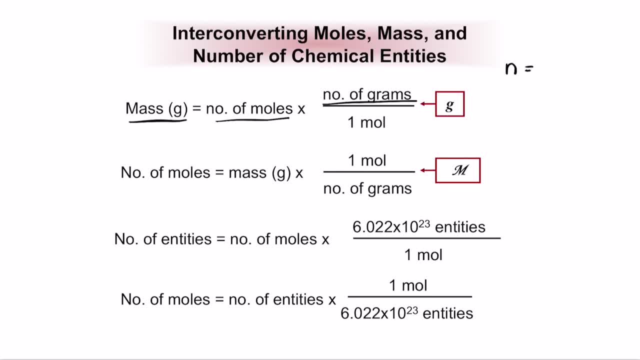 by these, generally given by the representation n, small, n, So n is given as mass by molar mass. So the number of moles is given by mass by the molar mass. The number of moles of a quantity is given by mass by molar mass. If you want to consider the number of molecules, 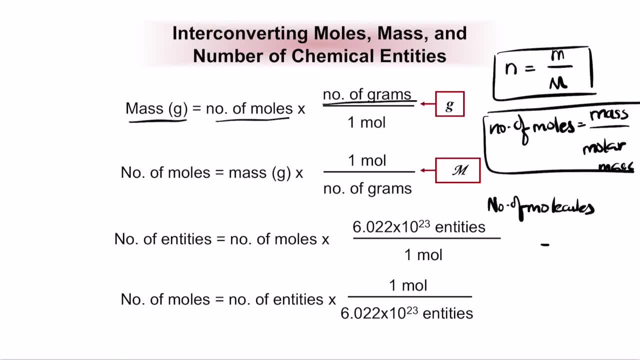 so multiply the number of moles with the Avogadro number. So that is where you get the number of molecules. and if you have the number of molecules and you want to calculate the number of moles, then we can calculate it by reversing the formula. So: 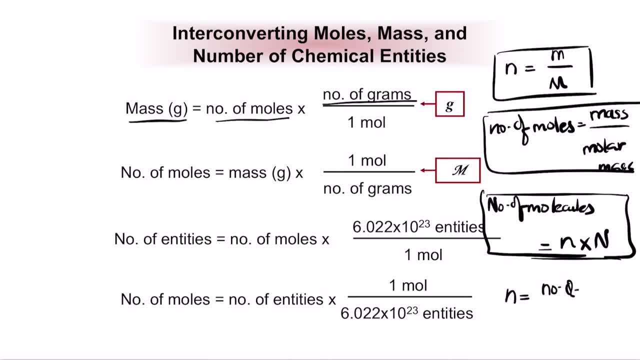 n becomes the number of entities over the Avogadro number. So these are the common formulas that we are going to end up using in this chapter. So make sure that you review these formulas just so that you remember. and main formula to remember is the number of moles is mass by molar mass. So this is the main formula to remember. 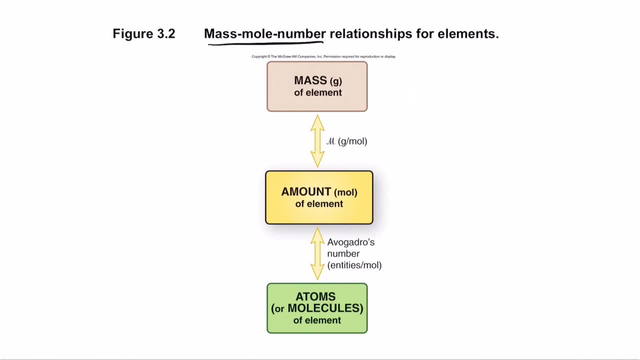 Now. so how do you mask more relationships, for elements change? So when you want to convert mass into moles, so we basically convert it by calculating, by multiplying it with the molar mass. So when you want to convert it into the number of moles of the substance, 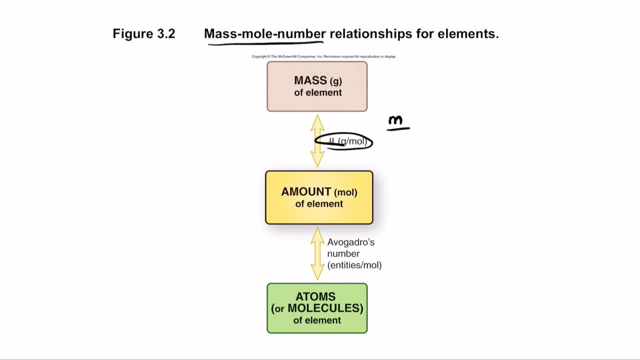 so divide it by the molar mass. So mass by molar mass gives you the number of moles. Now, multiplying that number of moles with the Avogadro number gives you the number of actual entities, or the atoms or molecules in that substance. So this is the idea behind the. 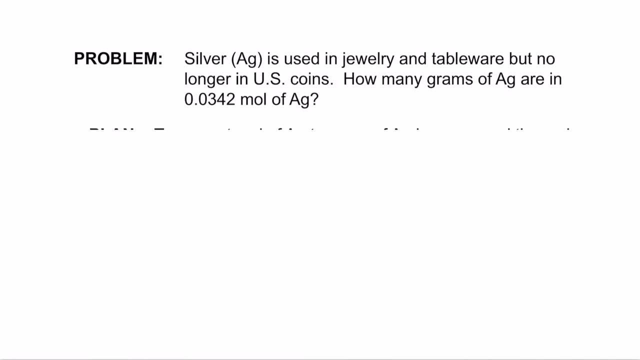 mass-mole number relationship for elements. Let's take a simple example. So let's take the simple example Here. so here they've given us silver. And don't forget that in AC, in this example, we've never shown this before. So the common formula is mass by molar mass. So they're asking us how many grams of silver? team, here is. 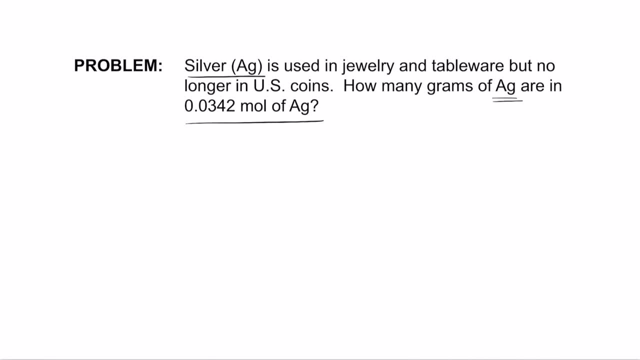 So let take a simple example. So here they've given us silver is used in jewelry and tablewear, but so bath off silver is used in 24 two my love silver. Now remember that 타 21 этом acabou 1ciones 얘기를 change�. 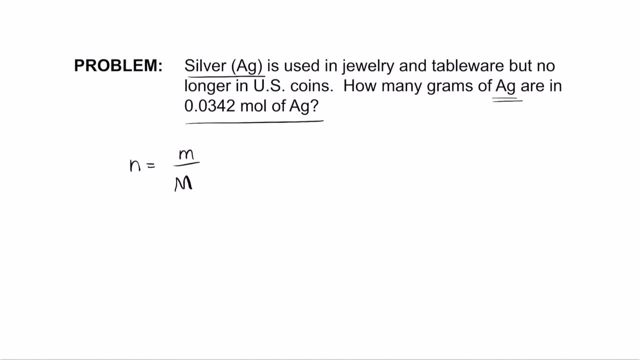 do matter. addemā pasht, uncomility, a number of moles. So they're asking us from extra grams and Paige red Kanglan as well. silver is there. so grams, remember that mass is represented by grams. molar mass is represented gram per mole. so now mass can be written as mass becomes number of moles into the molar mass. 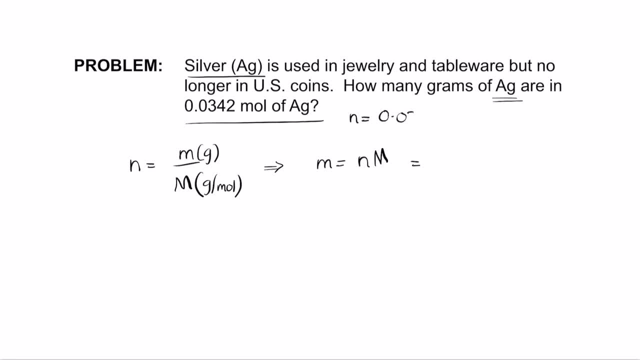 the number of moles is given in this problem, which is 0.0342 mole. so it becomes 0.0342 mole. but we do not know the molar mass, so we need the molar mass of silver. so how do you find the molar mass of silver? so from the periodic table. 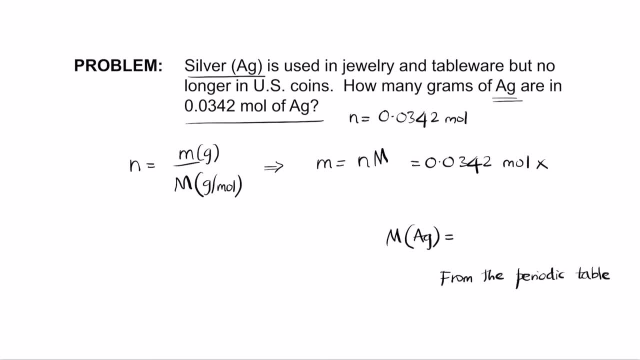 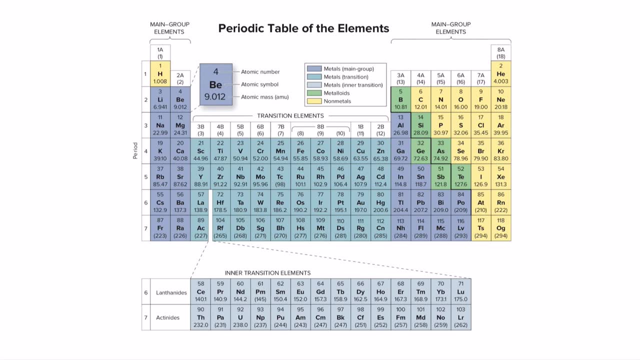 so let us look at the periodic table. so let us take a look at the periodic table. so from the periodic table we want to find ag. so where do you get ag here? so you have ag right here. so the value is given as 107.9, so let us use it. 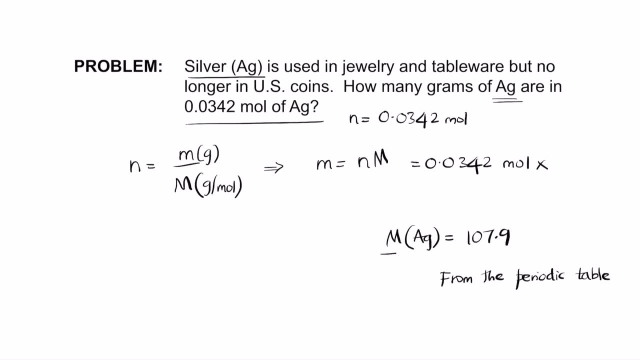 the value there, so that is 107.9. remember, this is the molar mass, which means you write it as gram per mole. so this is 107.9 gram per mole. so when you actually take out the units you still get the same unit in grams. so now you want to find the value. so that is 0.0342 times 107.9. 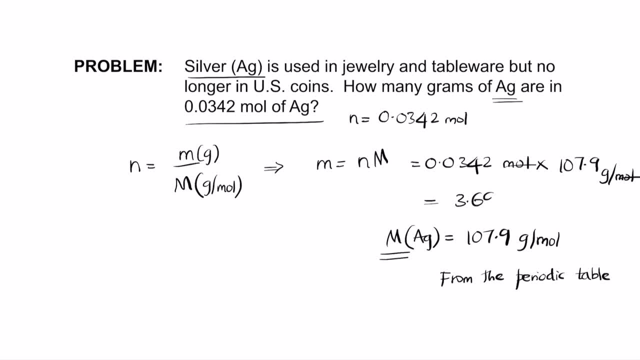 so that gives you a value of 3. 69018 grams. but remember the significant figures. we'll have to count the number of significant figures in the problem. so here the total number of the highest number of significant figures is four. so we have to use four significant figures. so when you want to use four significant 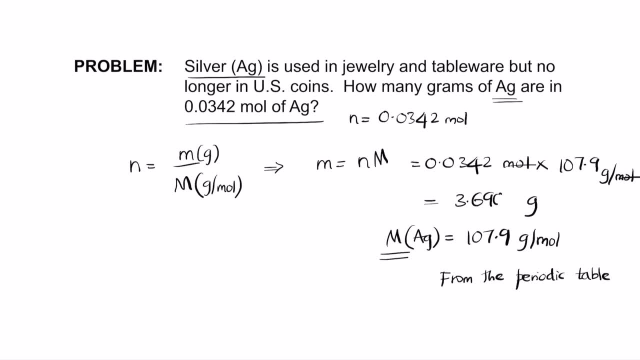 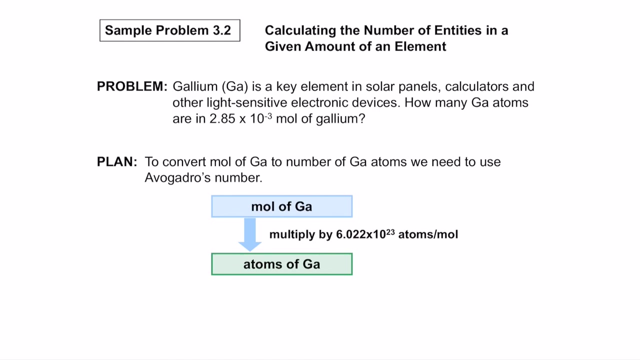 figures. so we have to eliminate the last two. so write it as 3.690 gram. so this is the mass of silver that is present in 0.0342 mole of silver. so this is how you can convert from one unit, one system, into another. so let us try another problem. so here they have, given you the problem. 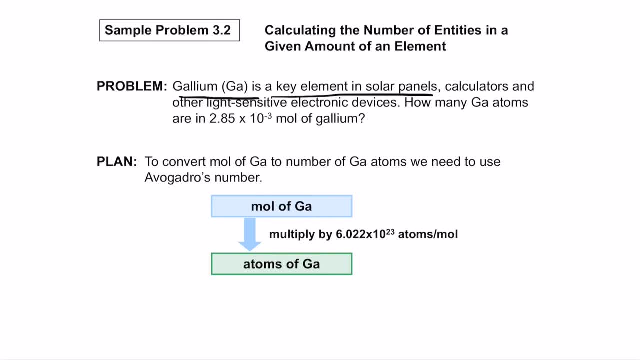 here. so gallium is a key element in the solar panels, calculators and other light sensitive electronic devices. so how many gallium atoms are present in 2.85 into 10 power negative 3 mole of gallium. so let us take a look at this problem. so the total number of moles n is given. 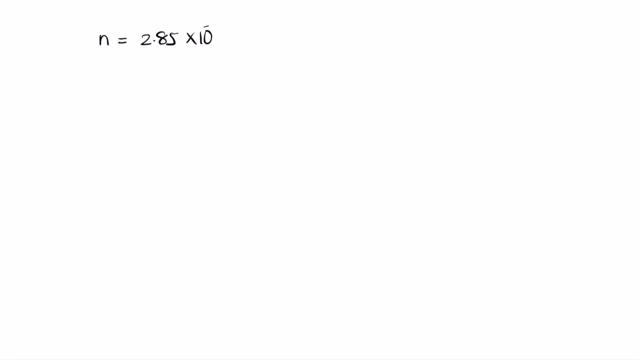 as 2.85 into 10 power negative 3 mole of gallium. so they are asking you to find the total number of gallium atoms. so remember the formula: total number of gallium atoms can be found as multiplying the number of moles with the Avogadro number. so the number of moles 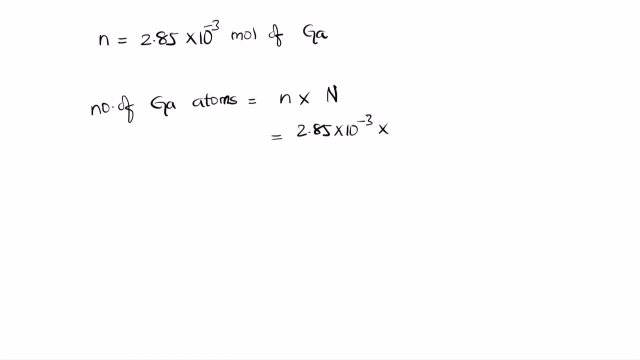 is 2.85 into 10 power negative 3 times the number of total. the Avogadro number is 6.022 into 10 to the power 23. so find the value. so if you multiply 2.85 with 6.022, that gives: 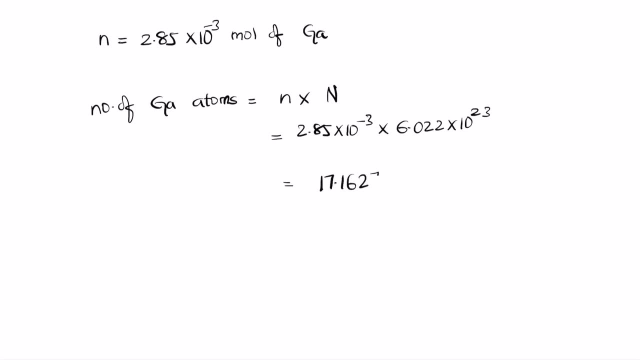 you an R value of 17.1627. but notice that the maximum number of significant figures you can have is 3, so round it off now. so when you round off this, you get 3 here. so when you round off 3, you get so 3. when you round it off, you get 6 here, so 6. when you round it off, this becomes 2. so the 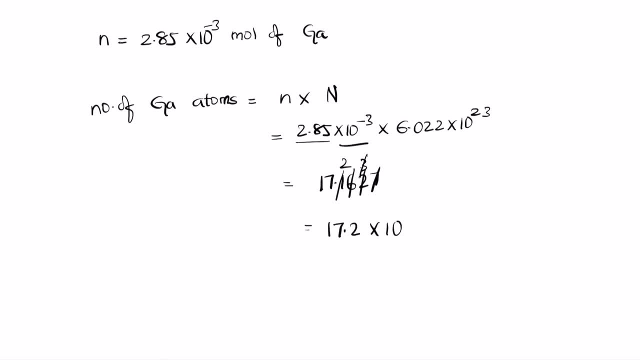 value should be 17.2 into 10 to the power. now this is 10 power negative 3 and 10 power 23. so you get this number one one side this way. so you get 1.72 into 10 power 21. so if you want to do it, if you, 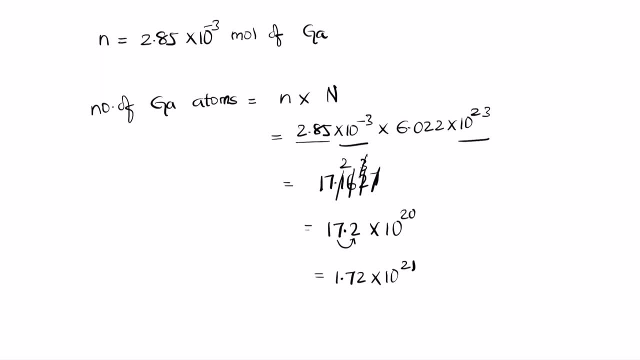 don't want to do it manually, you can try doing it by using a calculator. so now this gives you the final answer. this is the number of atoms in this many moles of gallium. so this is the number of gallium atoms. so remember the formulas. I'm going to write them again. so the number of moles: 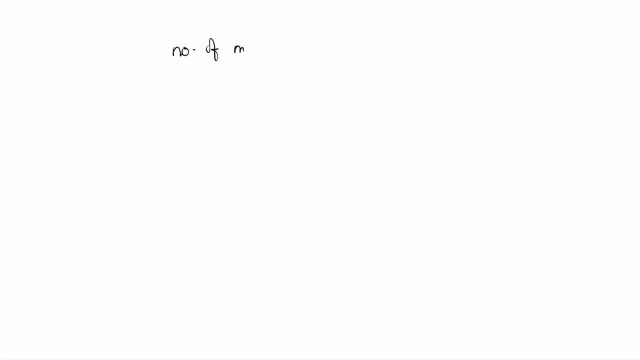 n is given by mass, small m over the molar mass uppercase M. so mass is in grams and molar mass is in Graham formula. so remember the formula's. the other one is the number of entities. so remember that whenever you change the term entities you can use it as atoms or formula formula, mass formula. 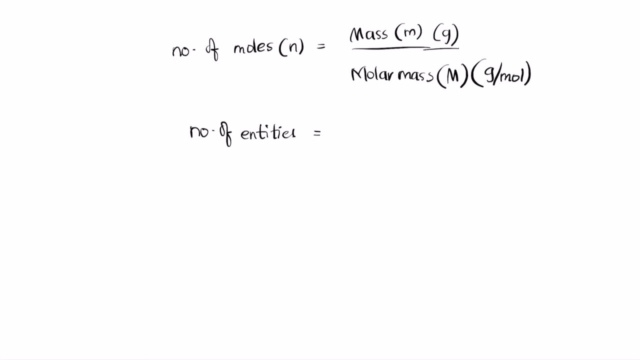 formula quantities, or you can use it as compounds as well. so the number of entities is the number of moles n times the Avogadro number. so, which is uppercase n, the value is 6.022 into 10 power 23 per mole. so remember these two formulas. so if you remember these two formulas, 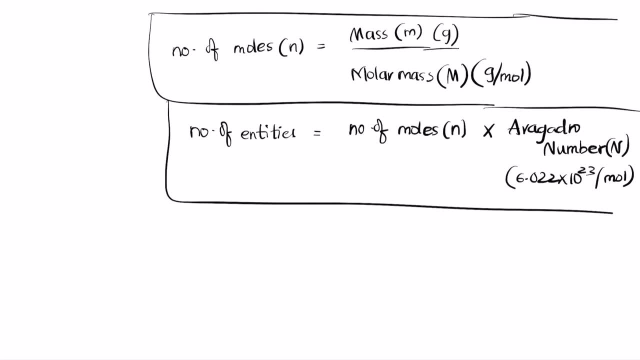 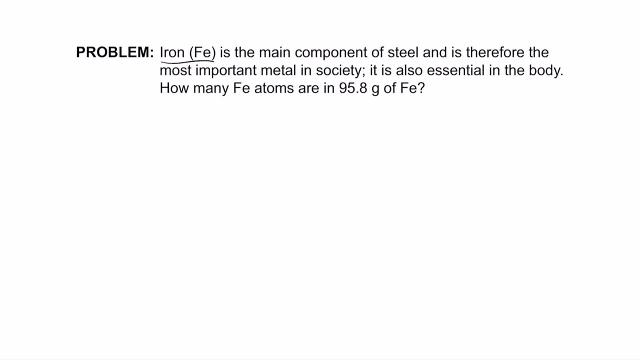 the entire first part of this chapter becomes easier. so let's try another problem. here you have iron, which is the main component of steel, is therefore the most essential metal in society, so it's also essential for the body. so they're asking you how many iron atoms are in 95.8 grams? 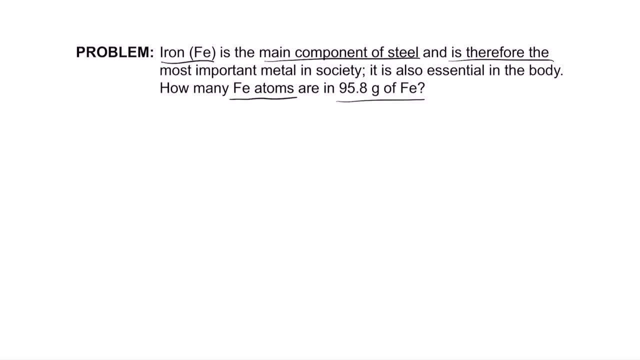 of iron. now pause the video right here and try to solve this problem. notice that they are asking two processes. so the plan here is to start connecting the two processes. so the plan here is to start connecting the two processes. so the plan here is to start connecting the two processes. so the plan here is to start connecting. 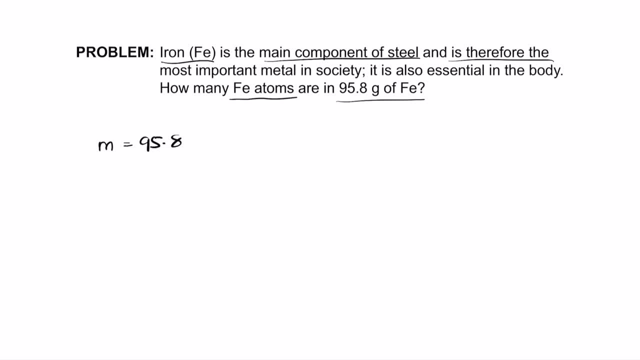 mass. so the mass is given 95.8 grams. so you're finding the number of moles first. so the number of moles is mass by molar mass. so first calculate using the periodic table, calculate the actual molar mass. so for your convenience I'm gonna write down the value. so the molar mass of iron: 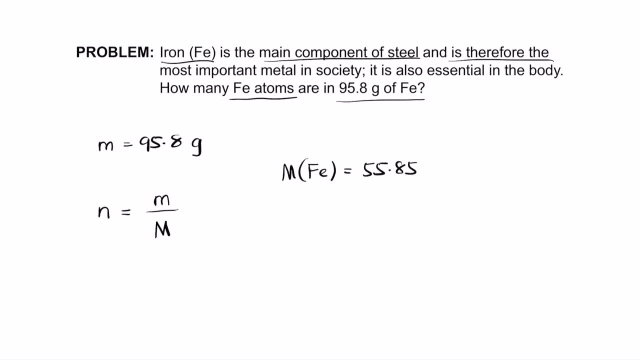 is 55.85 gram per mole. now, once you calculate the number of moles, they're asking you for number of iron atoms. so the number of iron atoms becomes the number of moles into the Avogadro number. so pause the video right here and try to solve this problem. 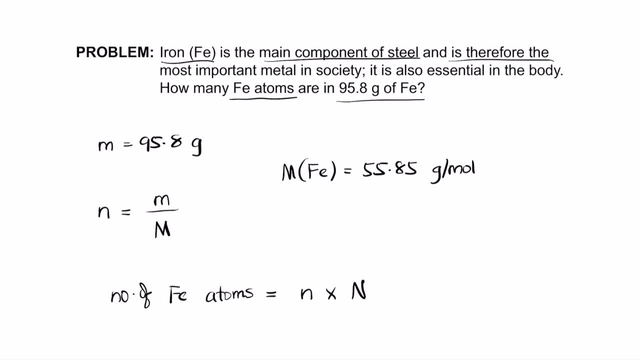 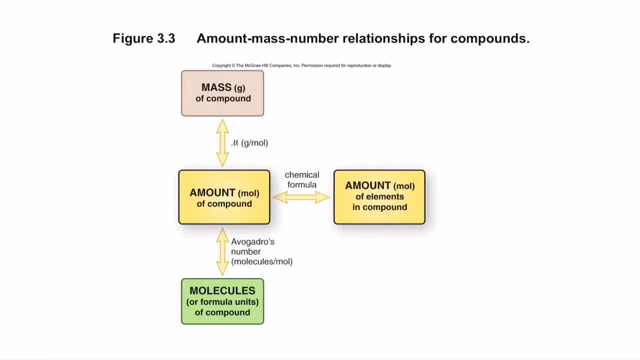 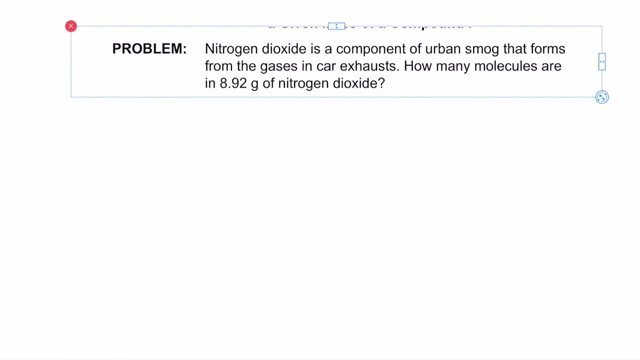 next, let's talk about amount, mass, number relationships for compounds. so what do you do when you have a compound rather than having a single entity or a single element? so let's take a simple example. so here we have a problem. so nitrogen dioxide is a component of urban smog. 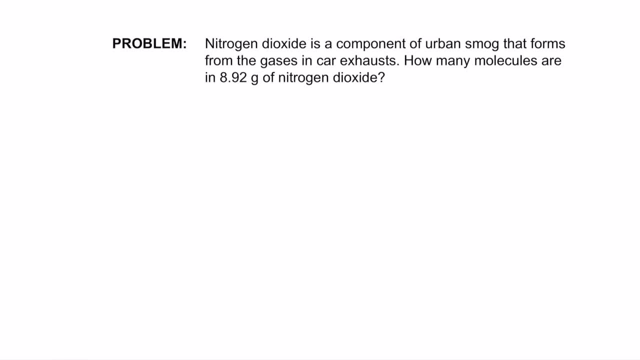 that forms the gases in car, car exhaust. how many molecules in? how many molecules are in eight point nine, two grams of nitrogen dioxide. so let me, let me try this one. so the mass is given. here is eight point nine, two grams. remember nitrogen dioxide, how to name it? nitrogen is an dioxide, so notice that die here, the die represent that there are two. 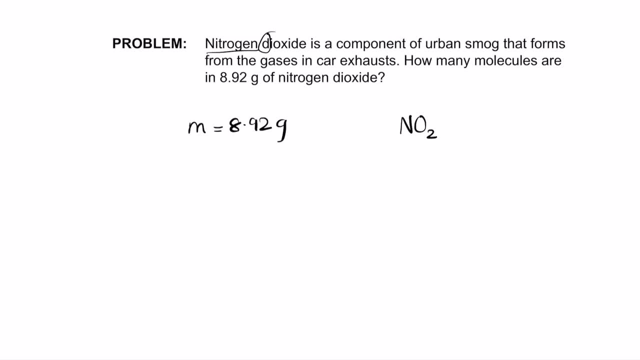 of them. so nitrogen dioxide no2. now we know the mass. now we want to find the molar mass. so the molar mass of an or two. so molar mass of an or two becomes so one times the molar mass of nitrogen dioxide. nitrogen plus 2 times the molar mass of oxygen, So 1 times So the molar mass of nitrogen. 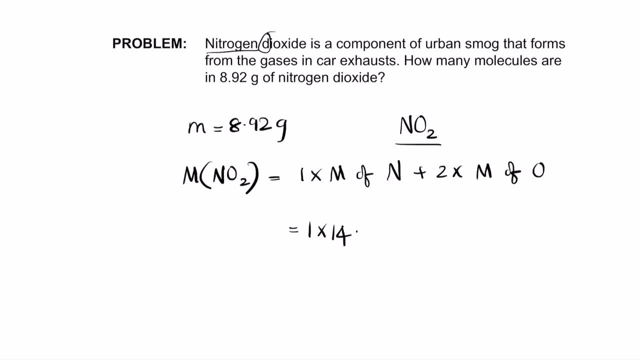 is 14.01.. So from the periodic table. So remember that these values I am writing are from the periodic table. So the molar mass of oxygen is 16.00.. So you have 14.01 plus 32.. 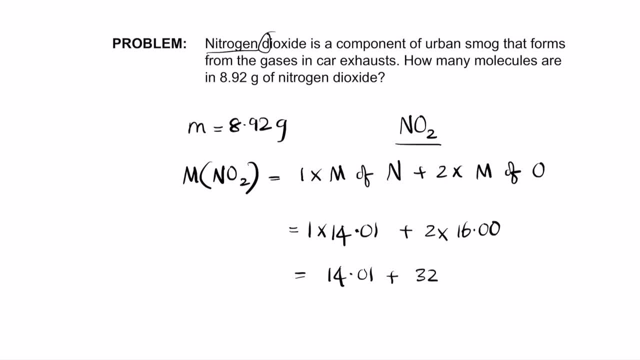 So 14.01 plus 32 gives you 46.01 gram per mole. Remember the units. Never forget the units for molar mass. Molar mass, always gram per mole. Now remember the part here. They are asking you for the number of molecules that are there, which means you have to first find the number of. 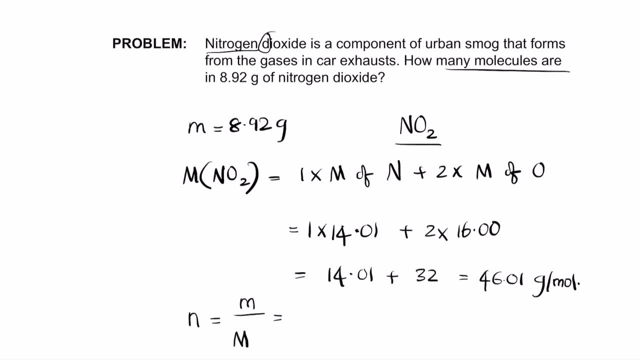 moles. The number of moles is mass by molar mass. Mass is 8.92 over molar mass is 46.01.. So 8.92 over 46.01.. That gives you a value of 0.194.. So notice that there are 3 significant 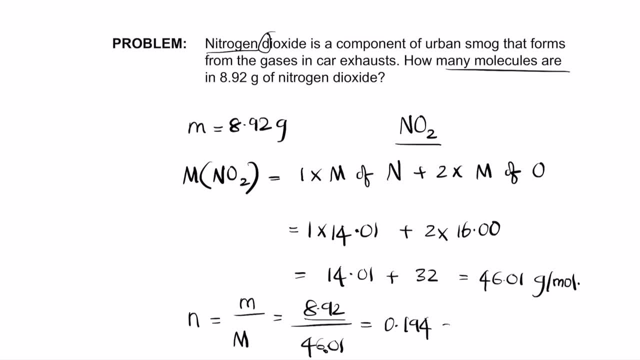 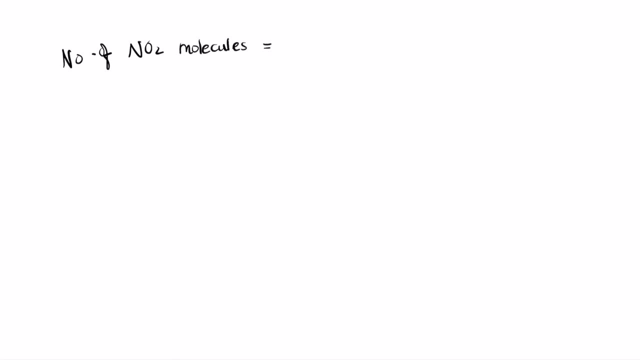 can be given by the formula: the number of moles times the Avagadro number. So the number of moles is 0.194 moles of NO2 times 6.022 into 10, to the power of 23 NO2 molecules. in how much 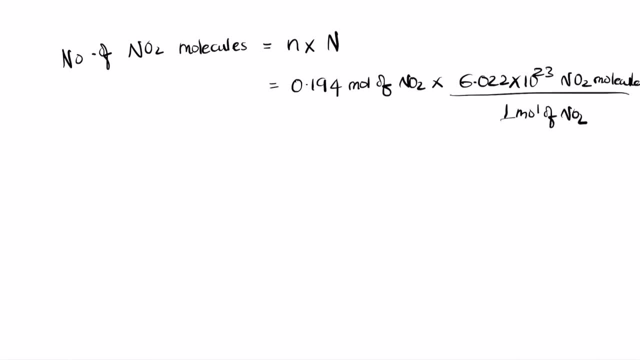 1 mole of NO2.. So molecules per mole, So mole and mole gone. So you have 0.194 into 6.022 into 10 power 23 NO2 molecules. So if I am using a calculator so that gives you a value of 1.17 into 10 to the power of 23 NO2 molecules. 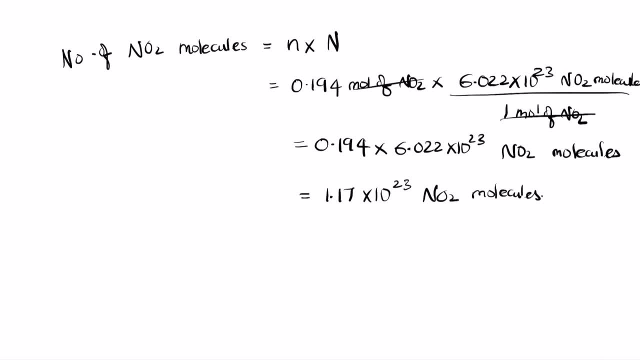 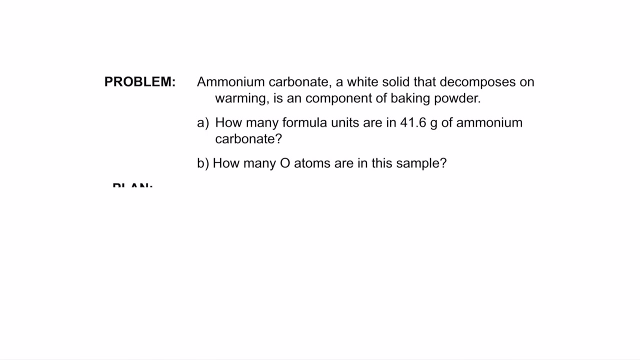 So this is the number of NO2 molecules in 8.92 grams of NO2.. So 8.92 grams of NO2 contains 1.17 times 10 to the power 23 number of NO2 molecules. So now solve this problem now. And they are also asking you, how many oxygen atoms are there here? 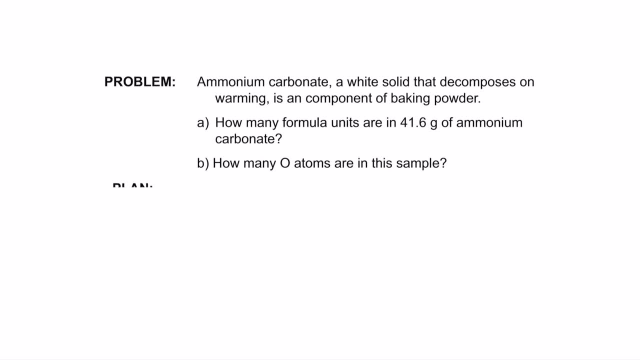 So this brings up the question: what is ammonium carbonate? So, if you remember the name, carbonate is CO3 and ammonium is NH4. So if you remember that both the charges is NH4 is plus, So CO3 is 2 minus and NH4 is plus, So shift the charges in the opposite direction. 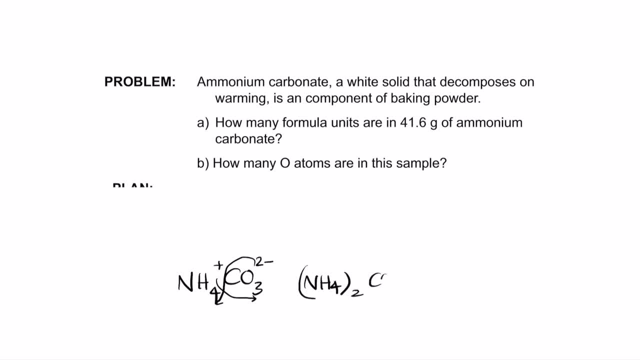 So you have NH4 taken twice CO3. So when you want to calculate CO3. The first one is the number of formula units of NH4. So that directly you can calculate it from the mass, just by the last method. Now I want to do the last one, which is B part. So B part represents the number of oxygen atoms. 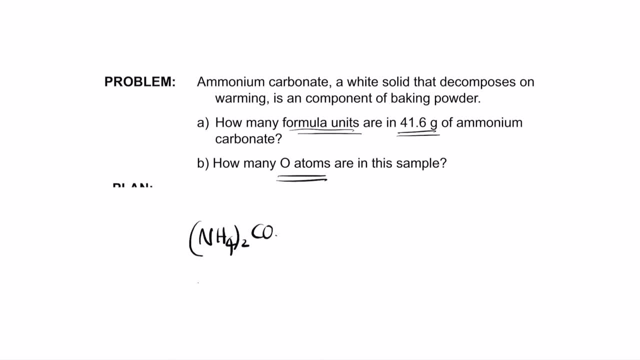 Notice that in each formula unit of ammonium carbonate, there is 3 oxygens. Use this ratio, which means that 1 mole of NH4CO3 contains 3 moles of oxygen, Which means that, whatever the number of molecules that you end up with, oxygen will be 3 times that number of molecules. 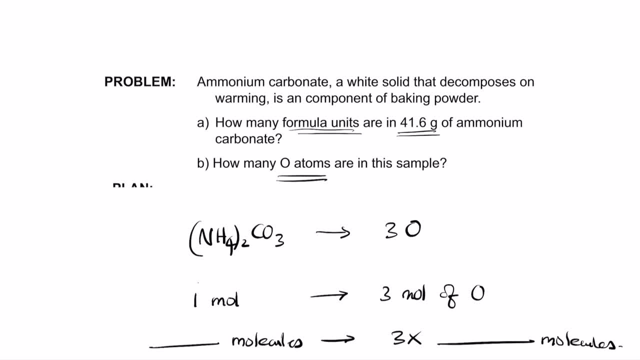 So remember the ratio here 1 is to 3 is the ratio, So, which means the molecules also will have the same ratio. So each formula unit has 3 oxygens. So 1 mole will contain 3 moles of oxygen. 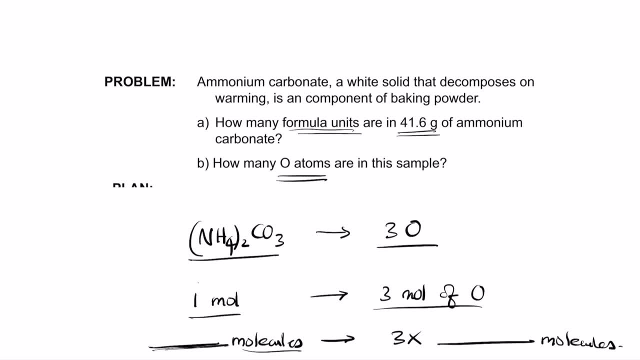 So whatever the number of molecules that you end up with, as the answer in the first part will be, so multiply 3 to it, that will be the number of oxygen atoms in the sample. So pause the video right here and try to solve this problem. 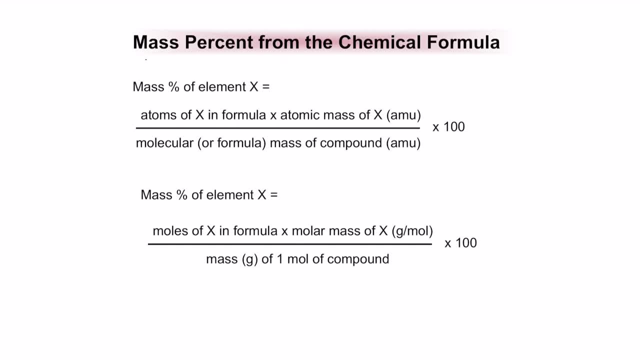 Next let's discuss the mass percent from the chemical formula. So every element will contain a certain amount that it contributes to the chemical formula. So that is what we are going to calculate as the percentage. So mass percentage, when you have an atomic mass will be atoms of the molecule, the number of atoms of a particular element in the formula. 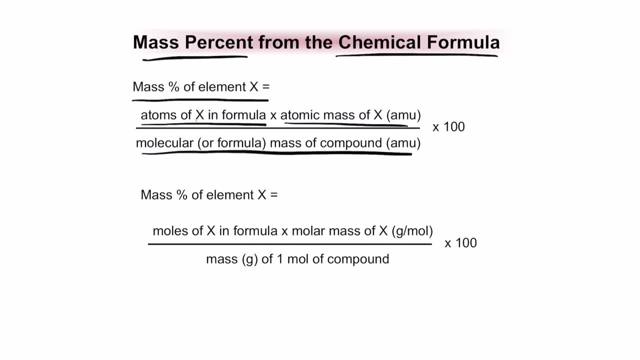 Times the atomic mass divided by the molecular mass of the component And when you want to have a mole, so the number of moles of the element in the formula times the molar mass of x divided by the mass of 1 mole of the component. 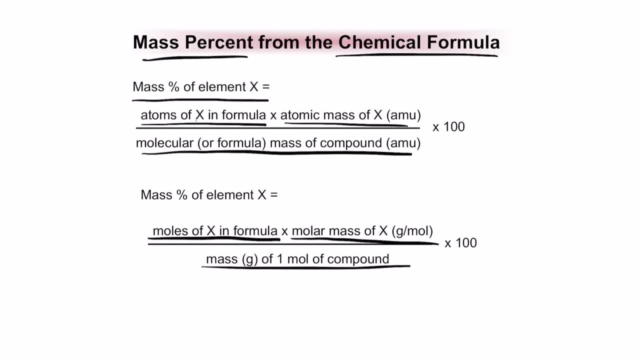 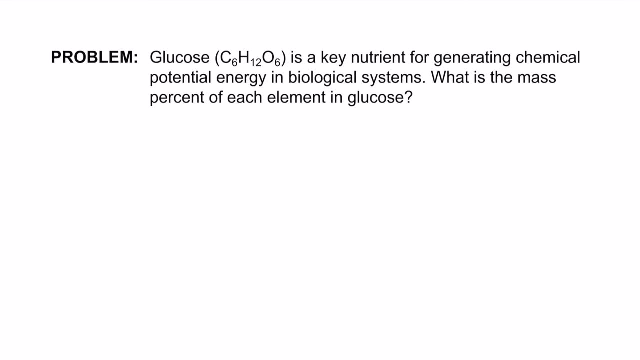 Now let's take a simple example and let's try to see if we can find out each of these mass from the values. So glucose is a key nutrient. So glucose is a key nutrient for generating chemical potential energy in biological systems. What is the mass percent of each element in glucose? 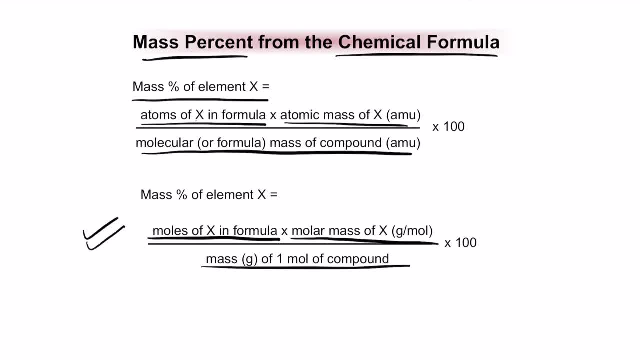 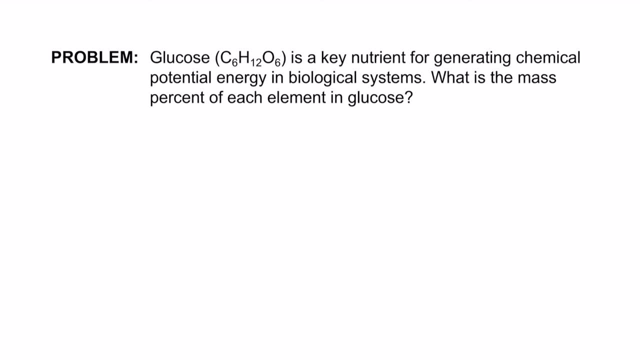 So, while we're using the second formula, because it's much easier, we don't want to confuse atomic mass and molar mass, So I'm going to use the second one. Now let's take the glucose here. So glucose is C6H12O6.. 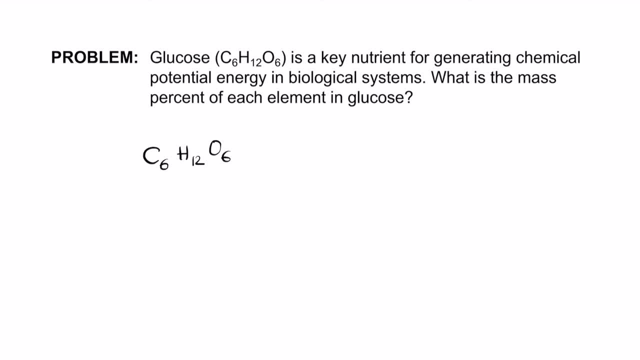 So for our understanding, let's consider that. So let's consider that there is 1 mole of glucose. So remember from the formula we are finding the mass percent of three elements. So we are finding the three elements here. The three elements are: one is carbon, the other is hydrogen, the last one is oxygen. 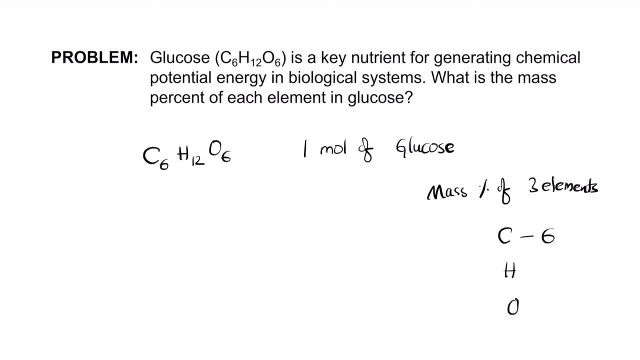 So there are 6 carbons, 12 hydrogens and 6 oxygens. So how do you find the mass percent here? So let's start with the mass percent of carbon, So the number of, so that becomes the number of moles of carbon. 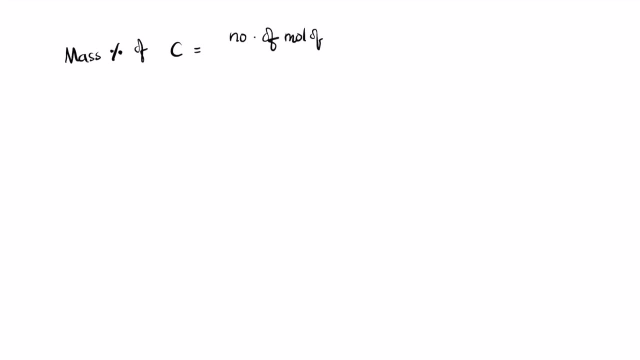 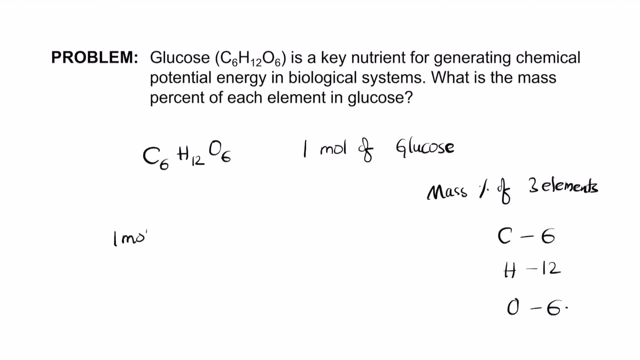 times the molar mass of carbon. So that becomes the number of moles of carbon mass of carbon over the mass of 1 mole of C6H12O6. So there are 3 things that we want to know. so notice that for 1 mole of glucose, 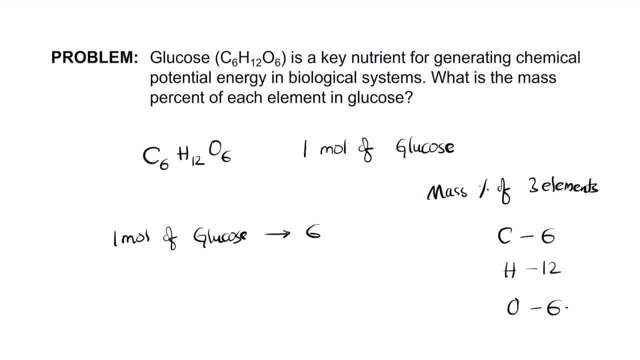 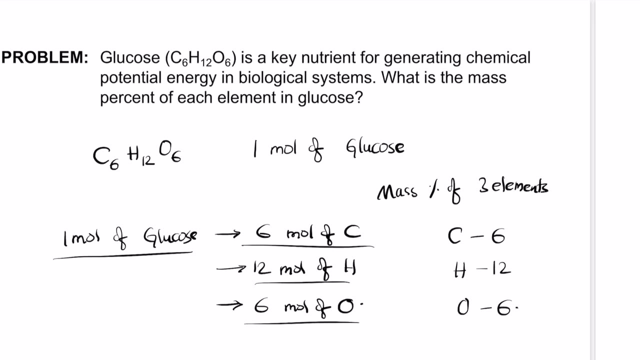 there is 6 moles of oxygen, sorry, 6 moles of carbon, 12 moles of hydrogen and 6 moles of oxygen. So this is the ratios that we are going to use in the formula. The other thing that we want to know is mass of 1 mole of C6H12O6.. So now calculate the. 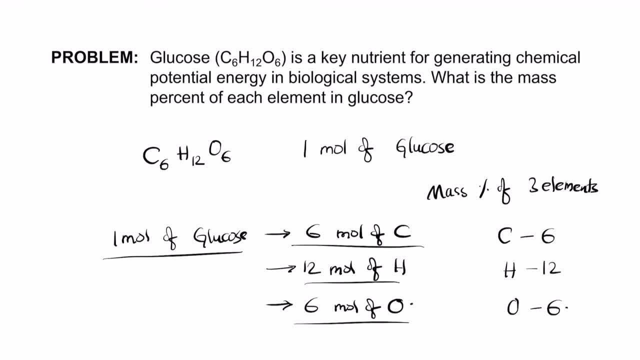 molar mass of C6H12O6.. So the molar mass of C6H12O6.. So the value is 6 times 12.01 plus 12 times 1.008 plus 6 times 16.. 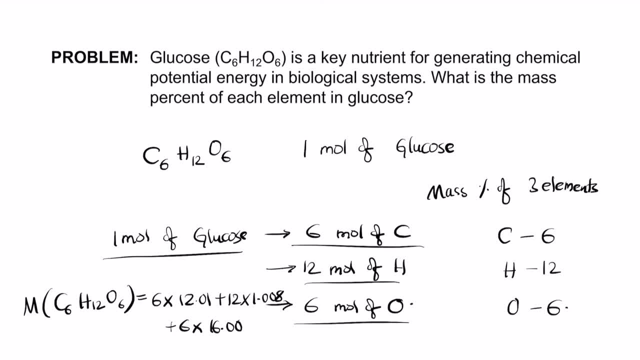 So 6 times 12.01 gives you 72.06 plus 12 times 1.008.. That gives you a value of 12.096 plus 12 times 1.08.. So 12 times sorry, 6 times 16.. 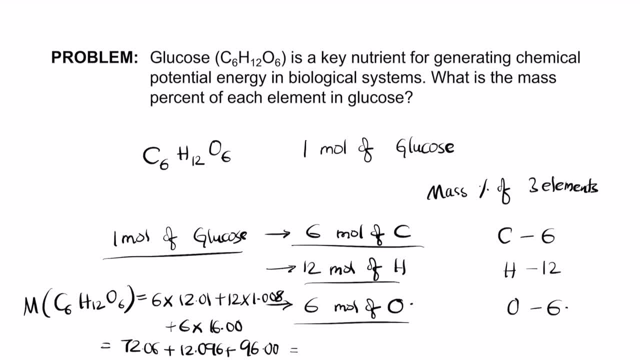 So that is 96.06.. So add everything up So that gives you a value of 180.156.. So notice that we need to have a total of 4 significant figures, So you have 180.. If you round off 6, you get 6 here, So 5 becomes 6.. So when you round, 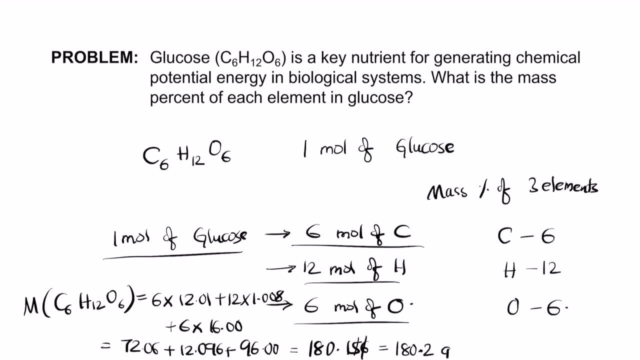 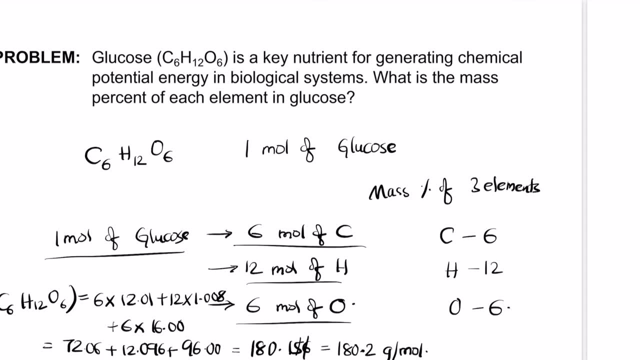 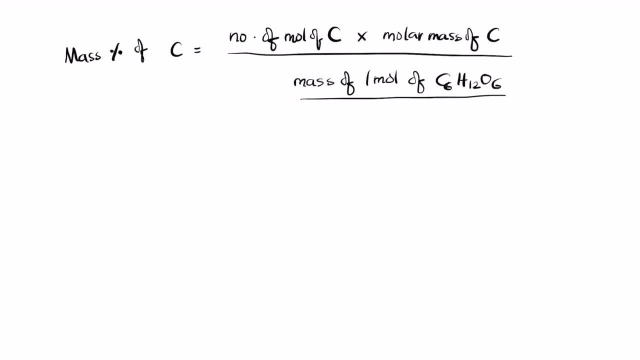 So 180.2 grams. Now the number of moles of carbon is 6 into the molar mass of carbon is 12.01. divided by the mass of 1 mole is 180.2 times 100. So when you calculate the value, So you have 6 times 12.01 over 180.2 times 100. So that gives you 39.988 percent. So we are close to 40 percent. 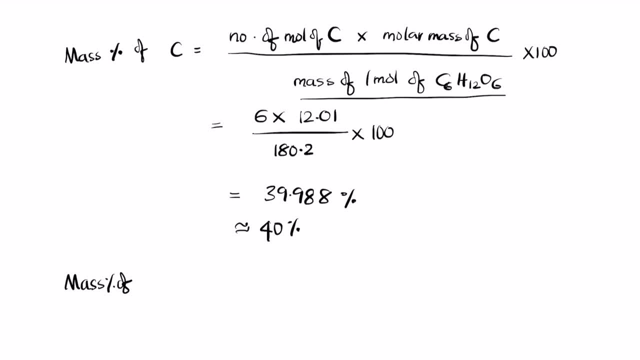 Next we want to find the mass percent of hydrogen. So that becomes the number of moles of hydrogen times the molar mass of hydrogen over the mass of one mole of glucose times 100. So that becomes 12.. Remember this: there are 12 moles of hydrogen. 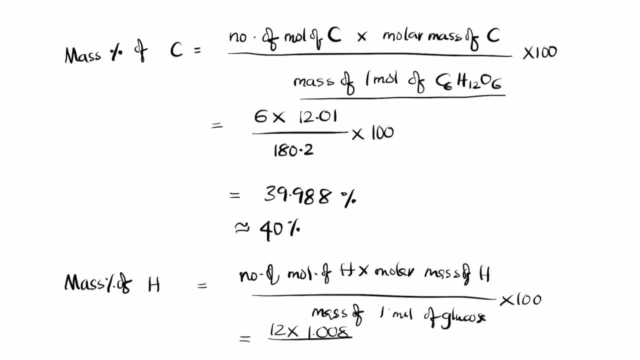 So 12 times 1.08, so from the periodic table over 180.2 into 100. So you have 12 times 1.08 over 180.2 times 100. That gives you 6.7125 percent. 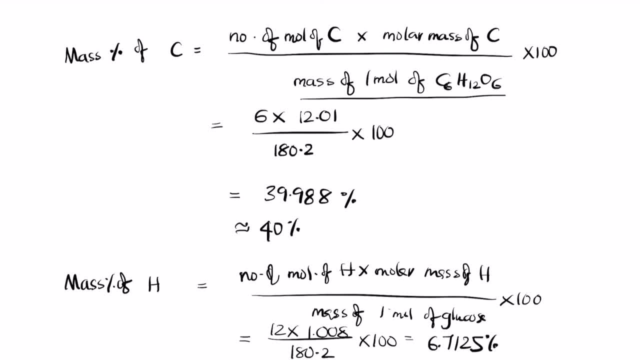 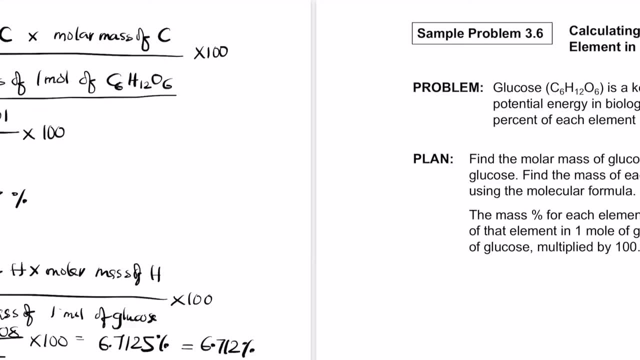 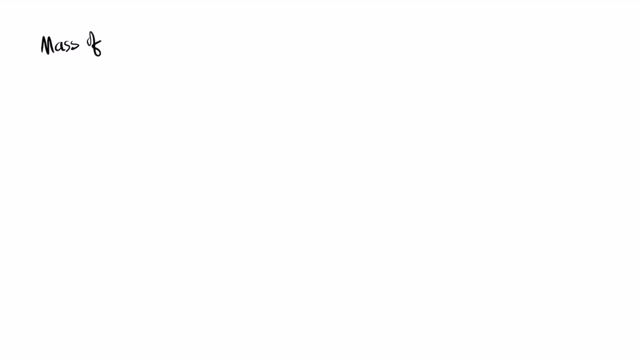 Okay, So the number of significant figures you want is 4.. So this becomes 6.7125 percent. Now the next one is the mass of oxygen, So the mass percent of oxygen. So oxygen, there are 6 moles of oxygen times molar mass of oxygen is 16.00 over 180.2.. 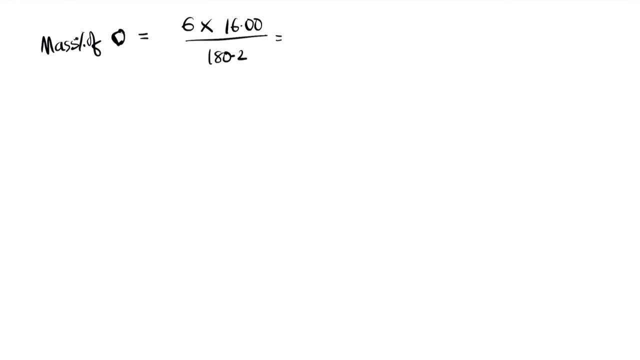 So 6 times 16.00, over 180.2, into 100. So that gives you 53.274.. So if you round it off you get 53.27 percent. So in a total, in total, the mass percent of each of these elements. 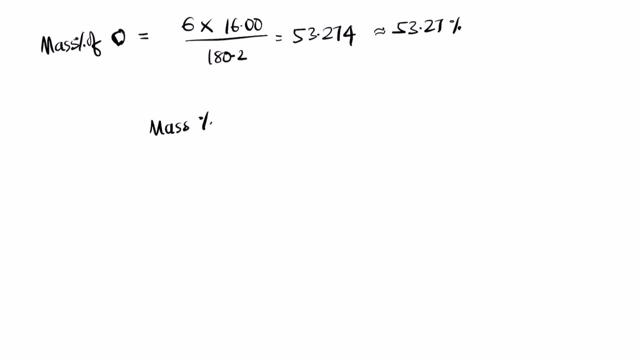 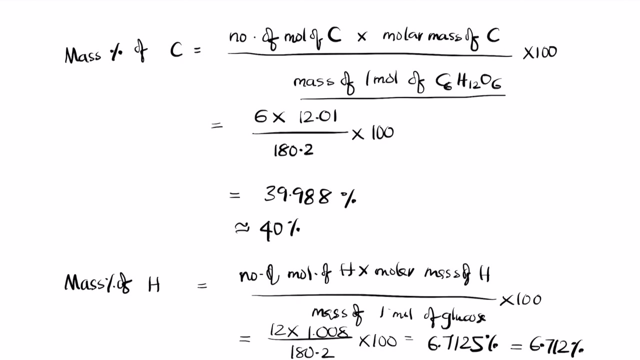 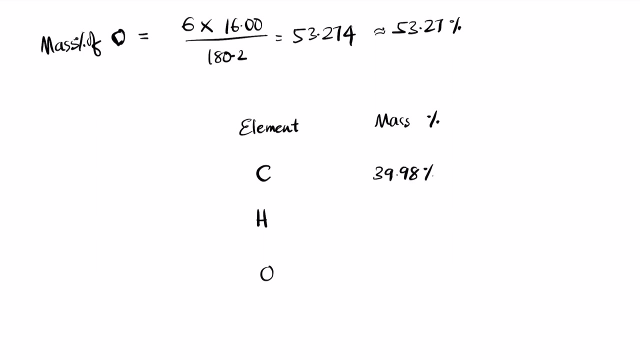 So let me write it as a small Jeremiah, Because it has numerical contributions. All right Now, as we now can see that this is a specific- discussions. Yeah, small table, so element. and the mass percent, so carbon, hydrogen and oxygen carbon has 39 point, so carbon in total has thirty nine point, nine eighty percent. 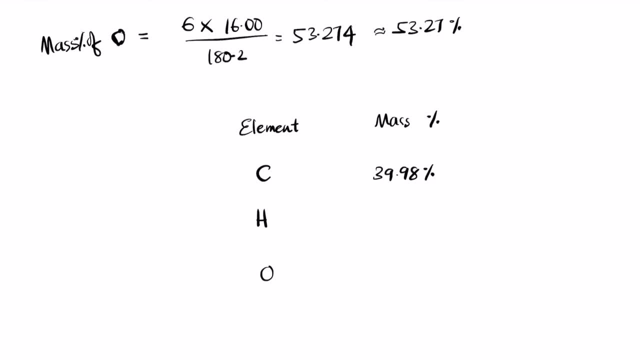 hydrogen has a total of six point seven one, two percent and oxygen has fifty three point two, seven percent. so if you end up adding all of them you should get a hundred percent. that's the idea behind the mass percent here. so this is in c6 H 2 by 06. so this is the problem. 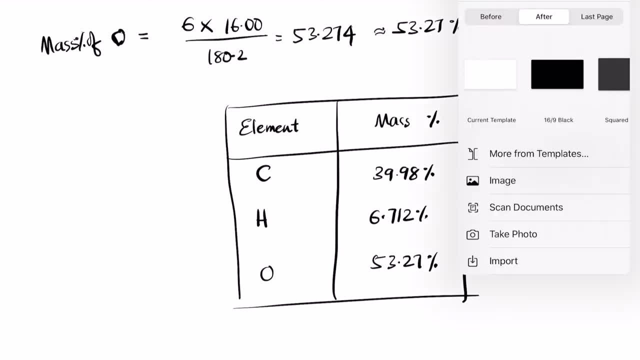 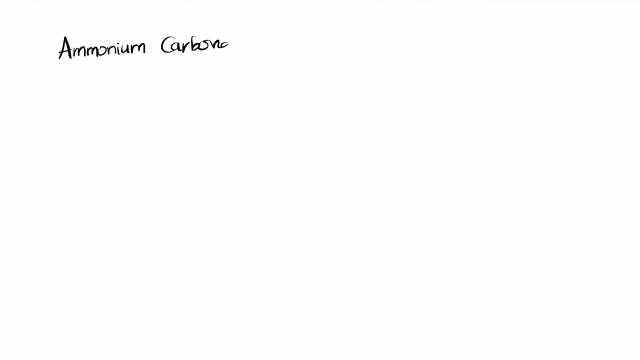 now. so now try an example. so try ammonium carbonate. so ammonium carbonate is nh4 taken twice, so thream. so if you want to calculate the, so try to calculate the mass percentage of each. I'm going to write all the atoms. so there is nitrogen, hydrogen, carbon and oxygen. there are two. 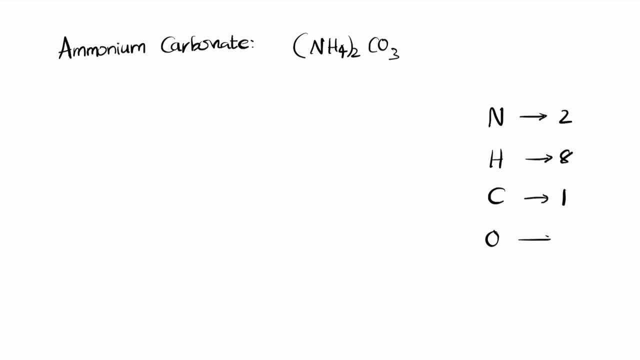 Nitrogen's, there is eight hydrogen's, there is one carbon. so text: here is the Kootenai 2. H2O comes in and says carbon đến t cried my. and three oxygens. so try to find the molar mass of. so try to find the compounds. 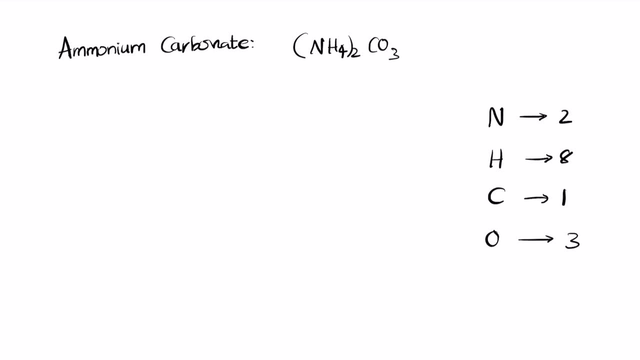 try to find the compounds mass percentage. so if you want, i can write the molar mass of nh4 taken twice. co3 ammonium carbonate is 80.05 grams per mole, so use the values. so pause the video right here and try to find the mass percentage of each of these elements. 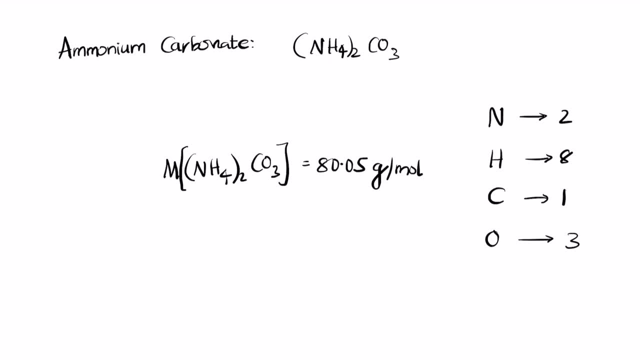 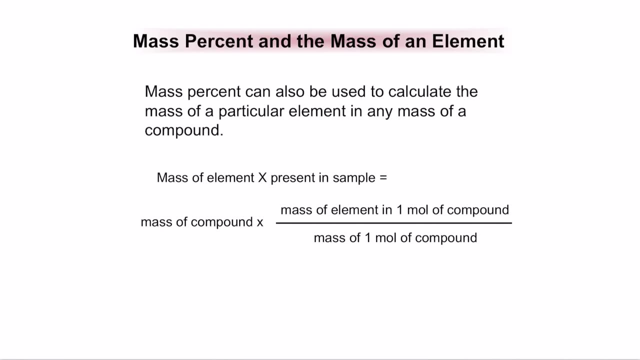 so now with the mass percent. one benefit of mass percent is it can help you calculate the amount of element for a given amount of mass. for example, if you take the formula mass of element, times, so the present in the sample, so the mass of the particular element present in the sample can be. 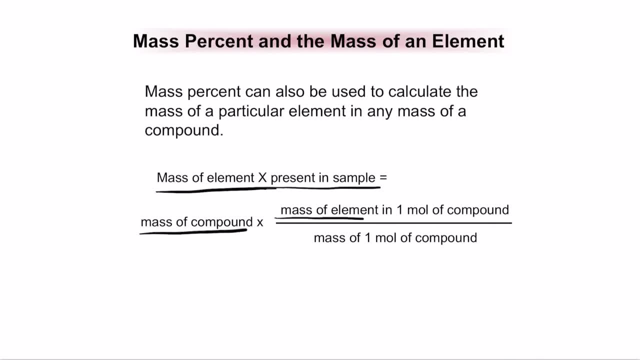 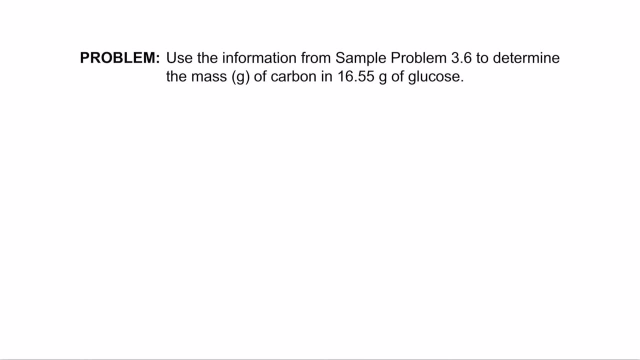 given by the mass of the compound, the mass of element in one mole, by the mass of one mole of the compound. So let us take a simple example of this. Let us take the same glucose example. They are asking you for the mass of. 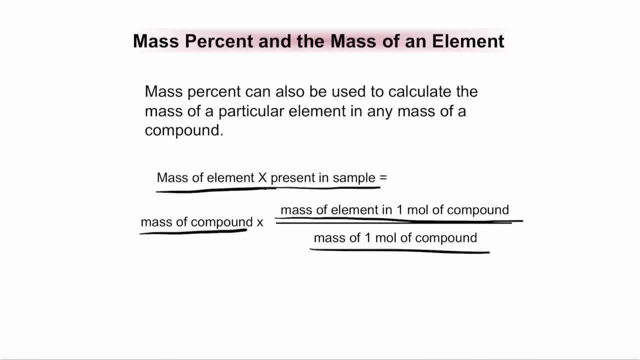 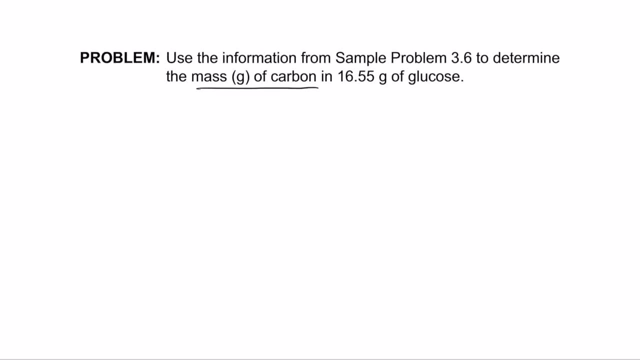 carbon. So remember the formula: mass of element present in the sample is mass of compound times mass of element over the mass of compound. So you have a total of. So they are asking you for mass of carbon can be given by the mass of glucose times the mass percentage of carbon in glucose. 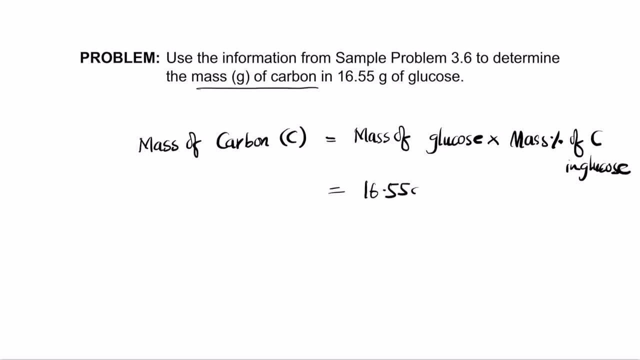 So the mass of glucose is 16.55 grams times the mass percentage of carbon. If you remember from the last problem, it is 39.99 percent. So 39.99. Remember percent, which means you have to write it by 100.. So calculate the value. 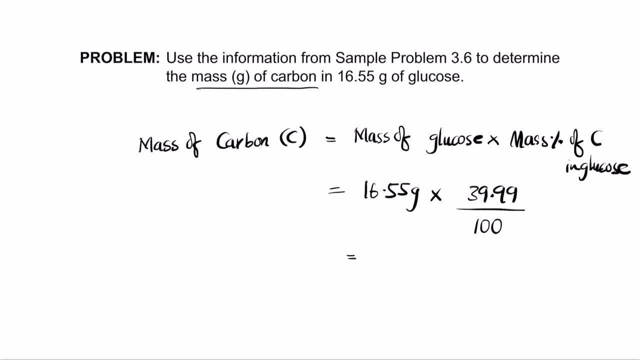 So you have 16.55 times 39.99 over 100.. So that gives you 6.618 grams of carbon. So this is how mass percentage can be used. So mass of any element can be multiplied with the mass of the compound times the mass percentage. 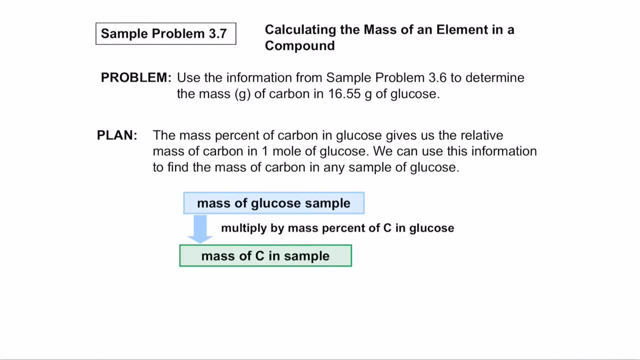 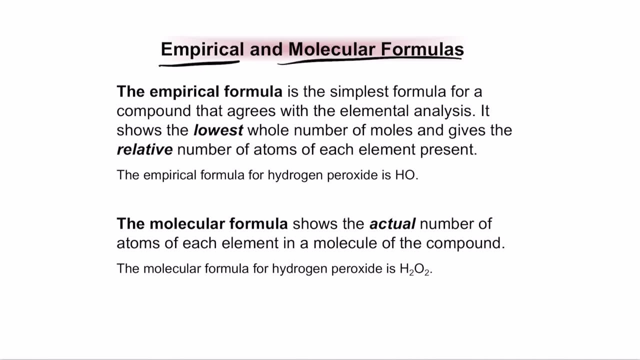 in that compound. So this is the simplest formula that you can use. Next let us go to empirical and molecular formulas. So what is the difference here? An empirical formula is the simplest formula for the compound that agrees with the elemental analysis. So it generally shows the lowest whole number of moles. 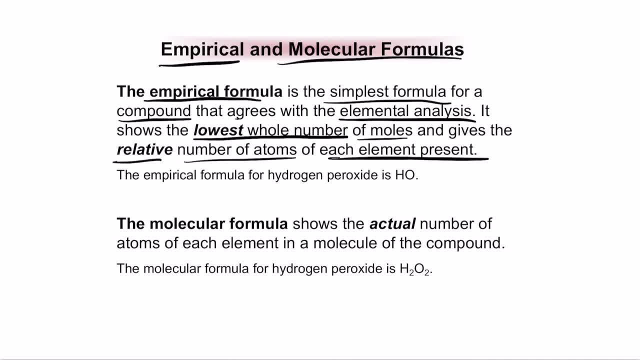 given and gives the Relative number of atoms of each of the compound. For example, when you take hydrogen peroxide, hydrogen peroxide originally is H2O2, but the empirical formula is HO, which means that this is the minimal number of atoms that are needed to form that compound and agree with. 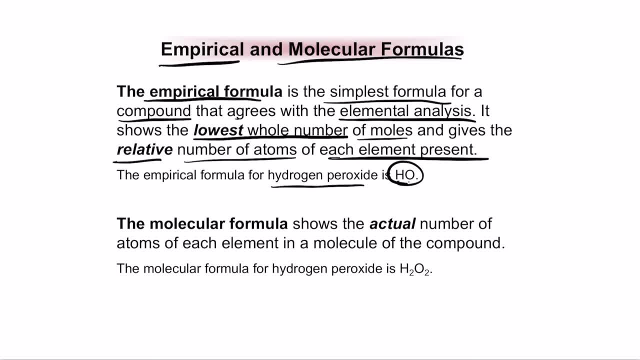 the elemental analysis. What is the molecular formula? Molecular formula is the one that shows the actual number of atoms in each element in a molecule or a compound right. So, for example, the molecular formula for hydrogen peroxide now becomes H2O2.. 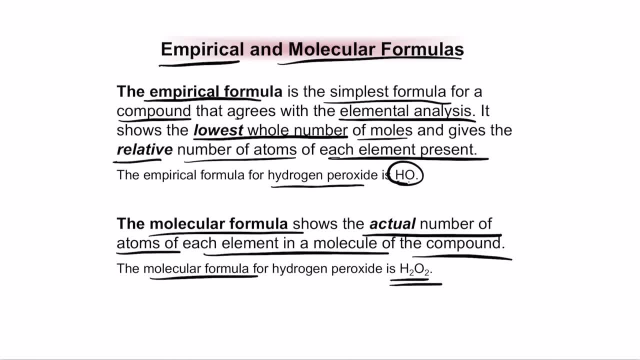 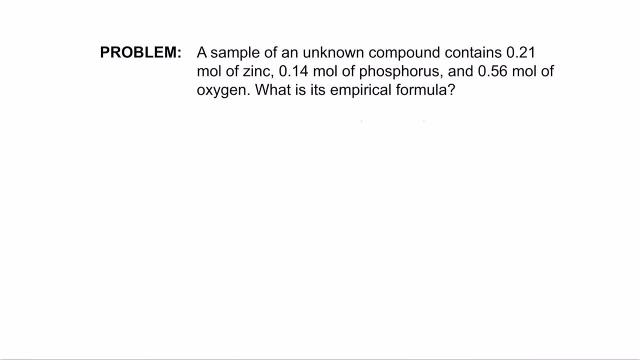 So you take out the common ones first, So you bring it to the smallest number possible of each element. That is the empirical formula. In the molecular formula we bring it to the molecule's actual identity. So let us take an example. You have a sample of an unknown compound. 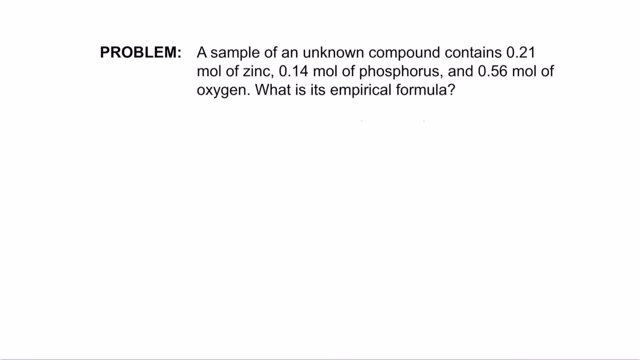 that contains 0.21 moles of zinc and 0.14 mole of phosphorus and 0.56 mole of oxygen. What is its empirical formula? So now let us, let us try how to determine the empirical formula. So what are the steps that we need to do First? so first, determine the mass in grams of each. 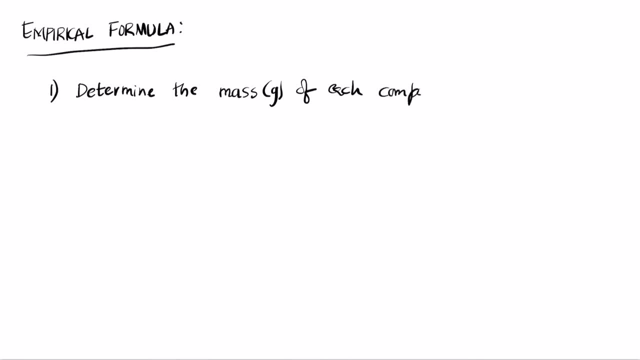 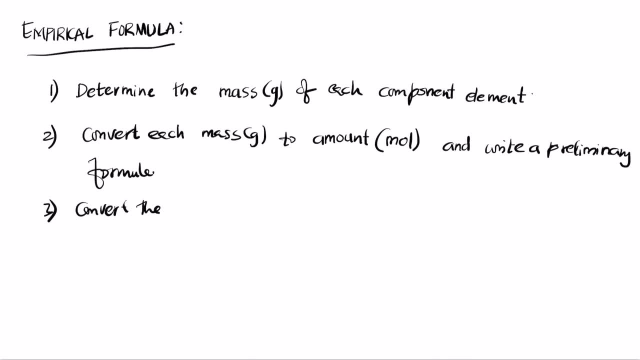 Third, convert mass into mole and write a preliminary formula with the smallest number. so, out of all the numbers, choose the smallest subscript number and divide it using that number. and finally, if necessary, multiply a small integer to convert any decimals into integers. right? so this is the the simplest way of doing it. so let's take a simple. 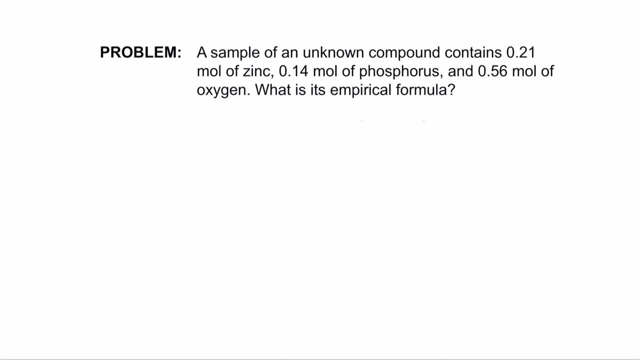 problem, and let's try to do it. so notice that the first step is already done, which means that they are already converted into mass and also converted into mole. so they have given us the actual mole of each quantity. so what do you do here is write down the element symbols. so zinc is zm, phosphorus is p. 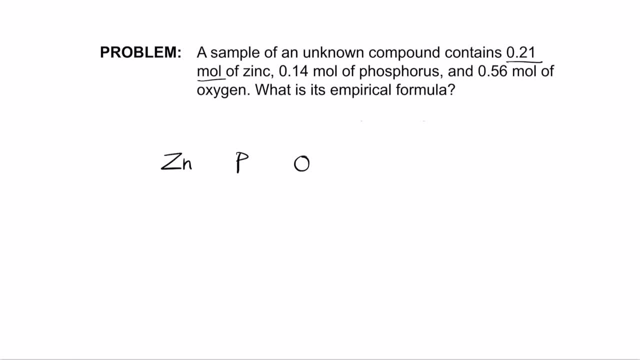 and oxygen is o and under the subscript. subscript is under the number write down the actual value of the number of moles. so 0.21, 0.14 and 0.56. so the first step is divide each subscript by the smallest subscript. so the smallest subscript here is 0.14. so 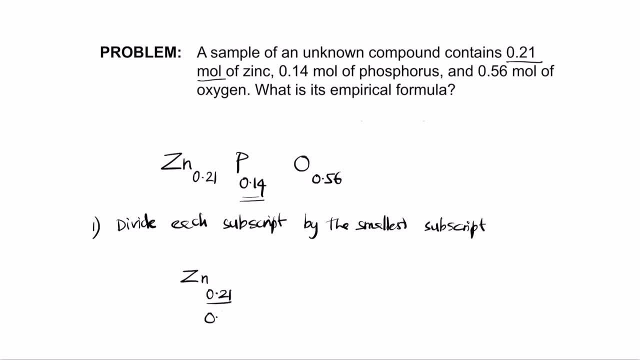 divide it with that, so you have 0.21 by 0.14, phosphorus, 0.14 by 0.14, oxygen, 0.56 by 0.14. so cancel it out. so cancel it out 0.14. this becomes four times, and when you cancel the first number, 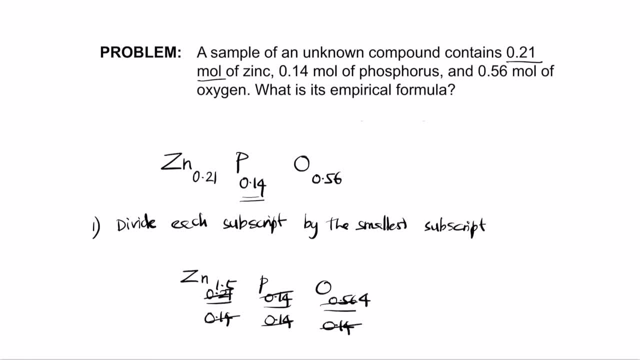 it is 1.5. so you end up with zinc 1.5, phosphorus 1, oxygen 4. now notice that 0.5 is not a fraction. the smallest number that you can multiply to it to get into an integer is to multiply 2. so when you multiply 2, so now multiply 2 to everyone. so zm 1.5 times 2, phosphorus 1 times. 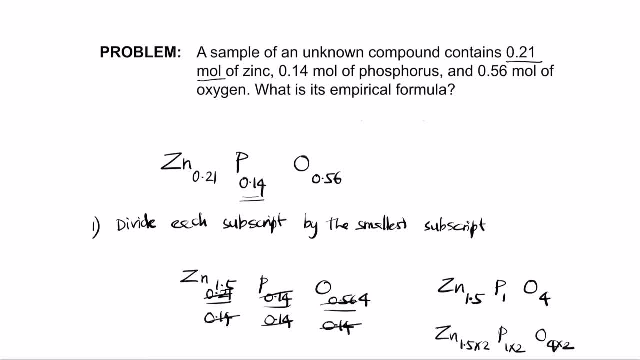 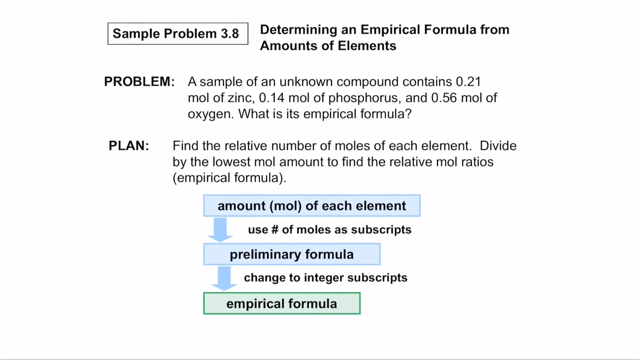 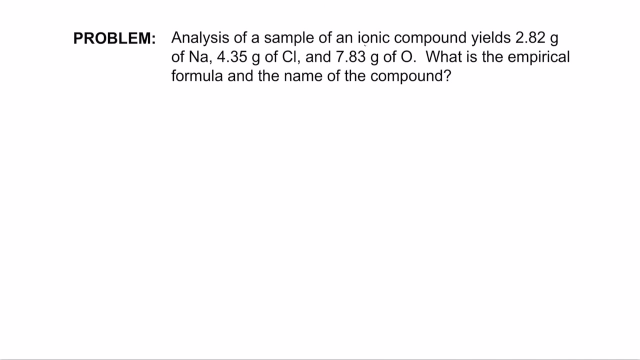 2 oxygen 4 times. so 1.5 times 2 gives you zm 3, phosphorus 2 oxygen 8. this is the empirical formula for the given compound, right? so hopefully the problem is clear. so let's try another example. so here you have analysis of an ionic compound so that yields 2.82 grams of sodium, 4.35 grams of. 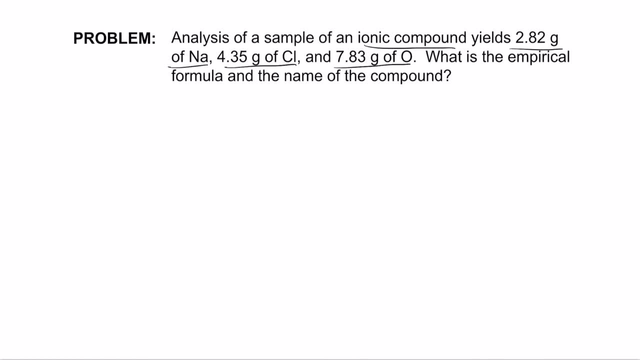 chlorine and 7.83 grams of oxygen. so they're asking you to find the empirical formula and name of the compound. so remember the first step: you convert the mass into the number of moles. so now we haven't find the number of moles of. 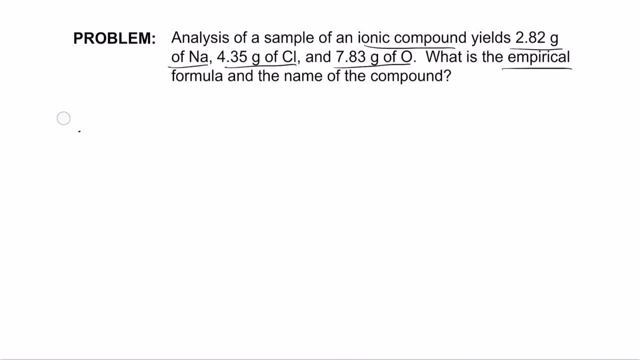 so let me write as the simplest version number of moles of sodium. that becomes the mass of sodium by the molar mass of sodium. so the mass of sodium is 2.82 grams. so 2.82 over the molar mass of sodium, if you can. if you take it from the periodic table, it is 22 point. 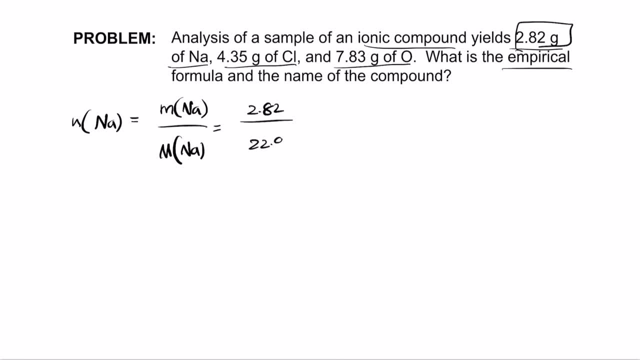 99, the value is 22.99 and when you calculate the value so that becomes 0.123. mole of sodium. next we want to find the number of moles of chlorine, so that becomes the mass of chlorine by the molar mass of chlorine, so mass of chlorine, the in the problem. 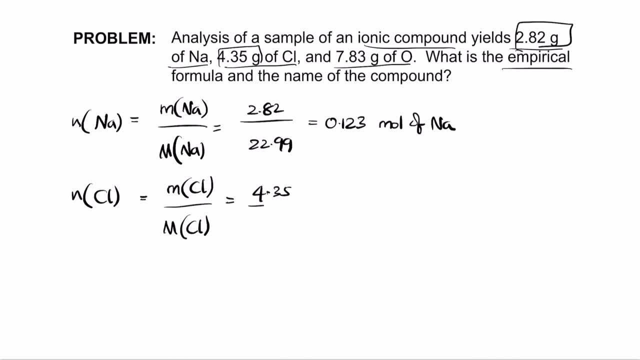 is four point three, five grams. so four point three, five. over the molar mass of chlorine is thirty five point four, five. so when you calculate total number of moles become zero, point one, two, three. mole of chlorine. next number of moles of oxygen, so the mass of oxygen. 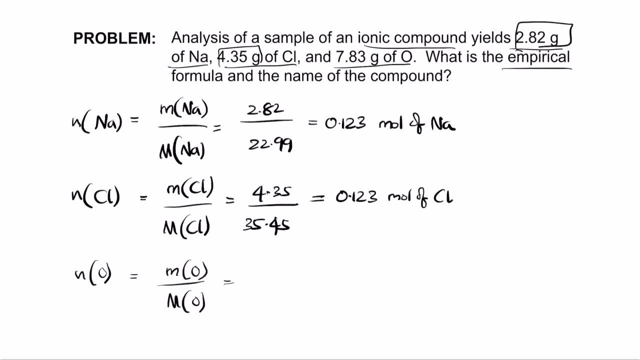 by the molar mass of oxygen. so the mass of oxygen here given as seven point eight, three grams over O, So that gives you a value of 0.489 mole of oxygen. So these are the final values that you have. Now what do you do in the next step? Write down the element and the number of moles in the 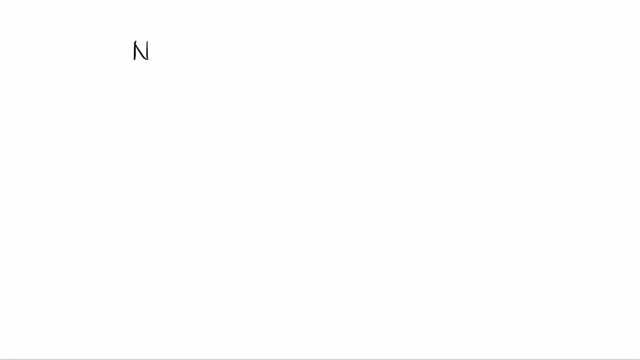 subscript. So sodium 0.123, chlorine 0.123, oxygen 0.489.. So in the next step, what do you do? Divide with the smallest one. The smallest one is 0.123.. So you have sodium 0.123 by 0.123,. 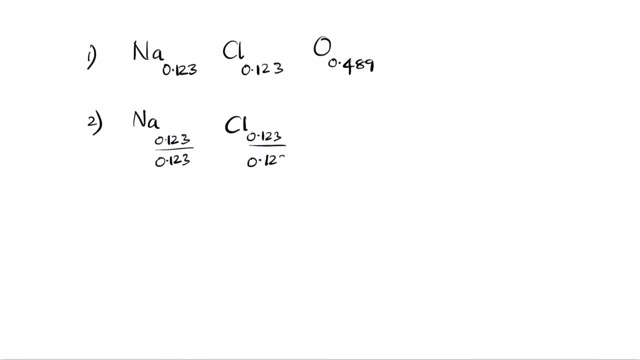 chlorine 0.123 by 0.123, oxygen 0.123 by 0.123, oxygen 0.123 by 0.123, oxygen 0.489 by 0.123.. So when you write down, you get sodium 1.00, chlorine 1.00,. 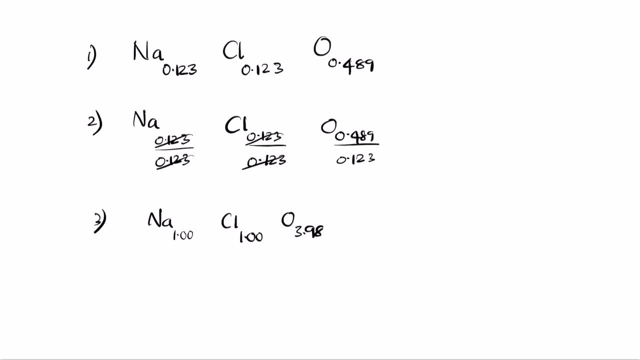 oxygen, you get a value of 3.98.. Now 3.98 is nearly close to 4. So you can round it off. So round off all the values, So you get Na1Cl1O4.. So 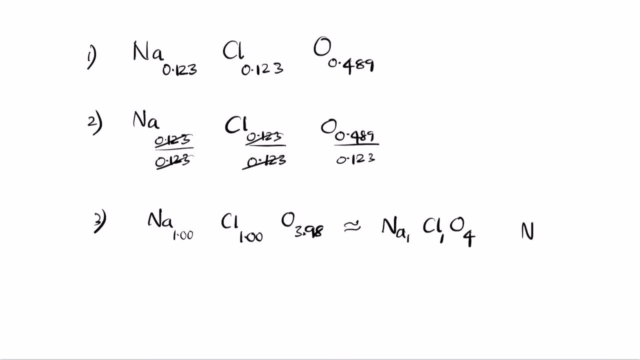 this is the formula, or you can write it as NaClO4.. So it is sodium perchlorate, If you remember from the last chapter. so the name is sodium perchlorate. So this is how you can start from mass and end up getting the final compound. 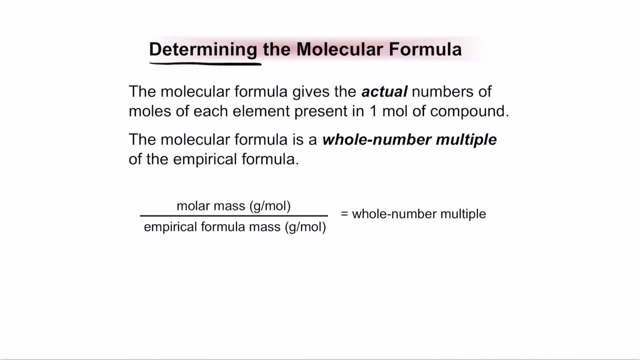 Next, next, try and find. let us try to find the molecular formula. So what we did now is try and find the empirical formula. So what, how do you find the molecular formula is just divide the molar mass of the given compound by the empirical formula mass. 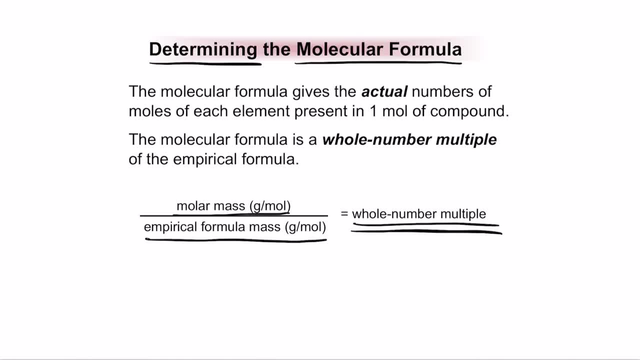 and you will get a whole number multiple. Multiply the whole number multiple to the empirical formula, that gives you the molecular formula. So the molecular formula is the whole number multiple of the empirical formula. So let us try this problem here. Notice that here. 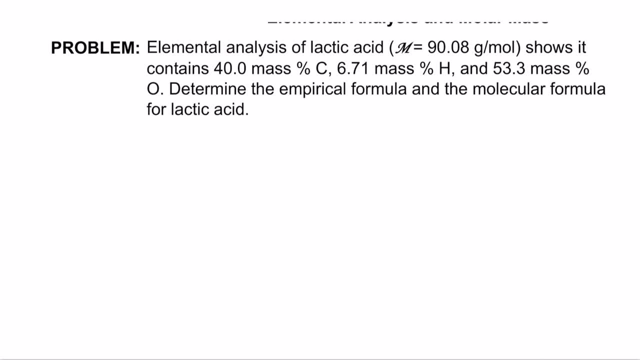 initially, all of them are in mass percent. So which means we have, we have to calculate the mass of each of these compounds first. So let us try from mass. So mass of carbon is they have given us the molar mass. remember that. So 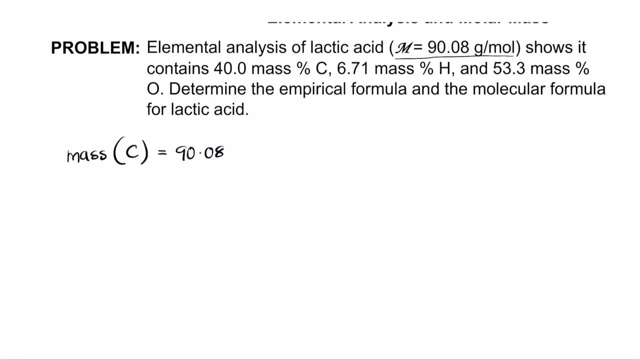 molar mass is 90.08 times the mass percent, 40 by 100. So that gives you a value of 40. So 40. So now let us try and calculate the mass of carbon. So you have 90.08 times. 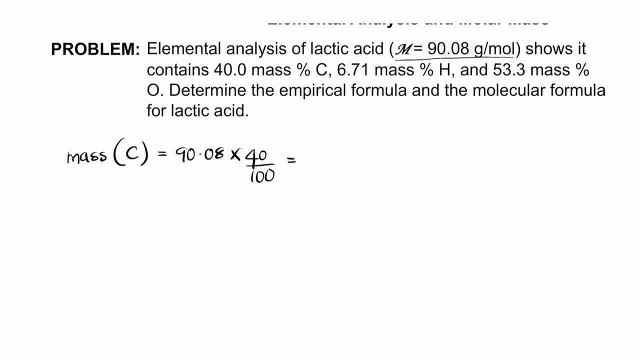 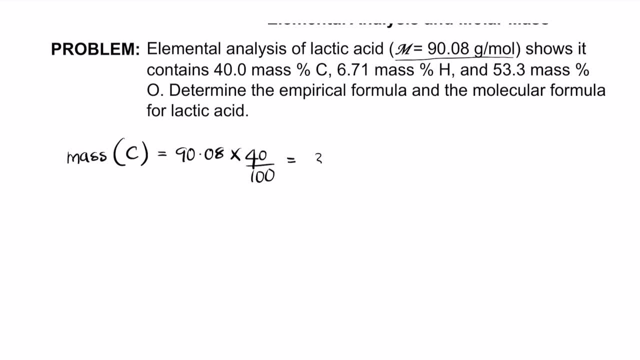 you a mass of 36.03 grams of carbon. Next, they are asking for mass of hydrogen that is 6.7 percent. mass percentage, that is 90.08 times 6.4 grams of carbon, So you have 90.08. 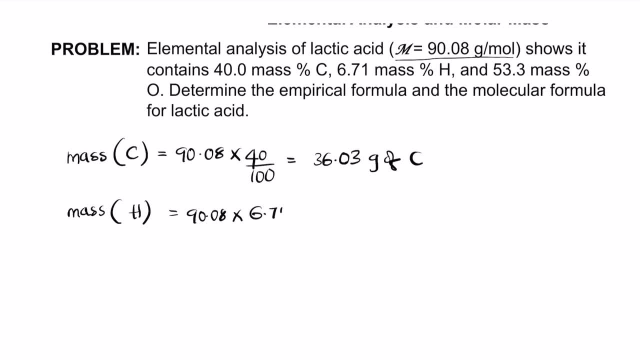 times 6.7 percent mass percentage, which isgetting 6.7 Byata. So that gives you value of 90.08 times. it shapes: ».071.. 0.4671.. so, So, So the value is 0.6.. 044 grams of hydrogen. Next, finally, the mass of oxygen. 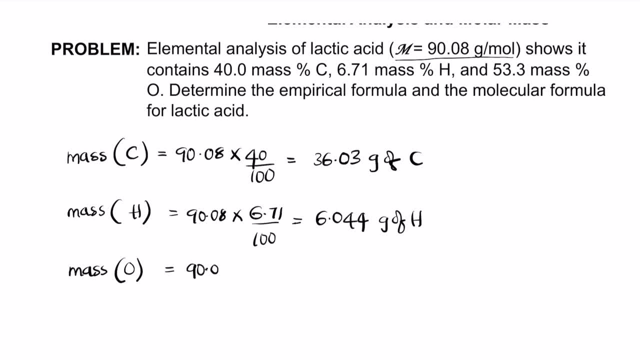 so that is 90.08 times 53.3, divided by one percent oxygen. and then for fr wheat, they, that's 50.W o g, that's YOU 100. so 90.08 times 0.533. so that gives you 48.01 grams of oxygen. so we have calculated all the. 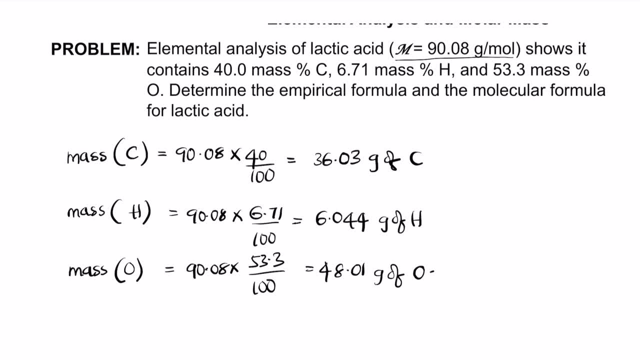 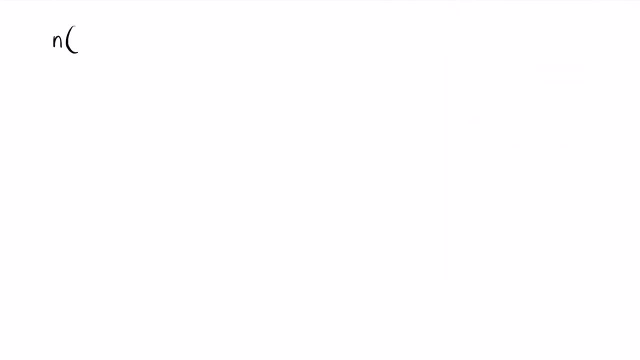 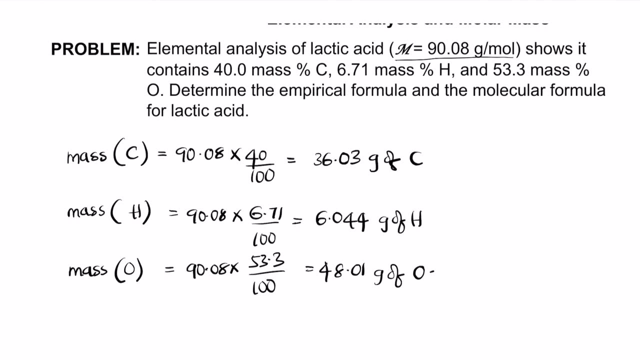 values that we need. next let's calculate the value for the number of moles. so remember the calculation of number of moles. so the number of moles of carbon is the mass of carbon by the molar mass of carbon. so the mass of carbon here is 36.03 grams. so 36.03 divided by mass. 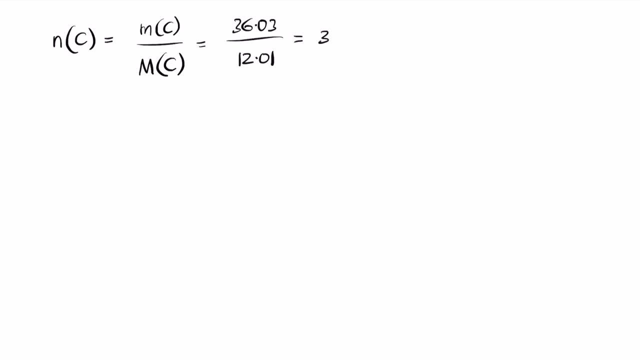 molar mass is 12.01, so that gives you a value of three point. so 36.03 over 12.01 gives you a value of three. so this is the number of moles of carbon. next number of moles of carbon is the number of moles of carbon. so this is the number of moles of carbon. 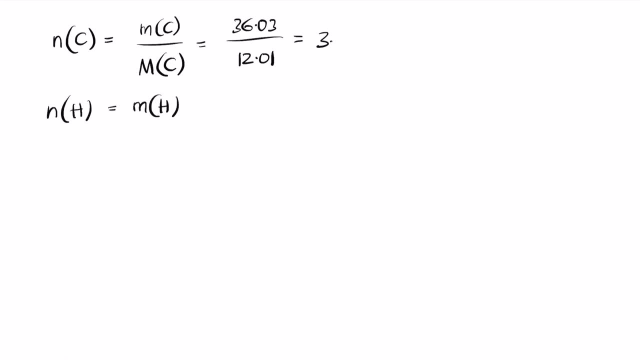 is the number of moles of hydrogen, and the number of moles of hydrogen is the mass of hydrogen by the molar mass of hydrogen. so the mass of hydrogen is 6: .044 divided by 1.08. you have 6.044 divided by 1.08, so that gives you a value 5.996, which is nearly equal to 6. next number ofol of oxygen is the mass of Tok cas n e of oxygen: 15960389. 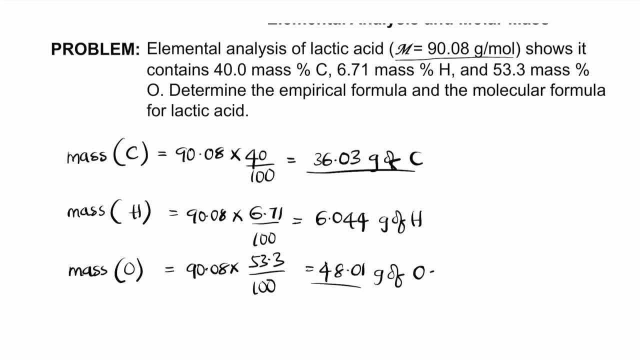 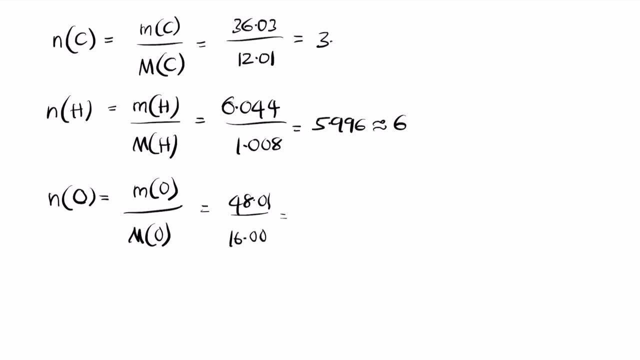 by the molar mass of oxygen. So the mass of oxygen is 48.01 divided by 16.00.. So 48.01 divided by 16.00 gives you 3.00.. So which is nearly equal to 3.. Now write it as a subscript. 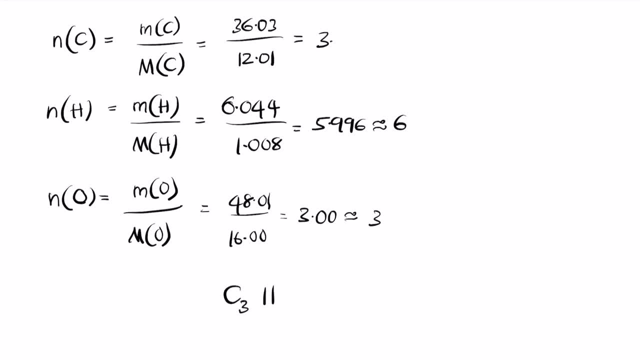 We have carbon 3, hydrogen 6, oxygen 3.. So the smallest number here is 3.. So you get 3 by 3, hydrogen 6 by 3, oxygen 3 by 3.. So 3, 3, 1, 3, 1s, 3, 2s, 3, 1s, So you get C1H2O1.. 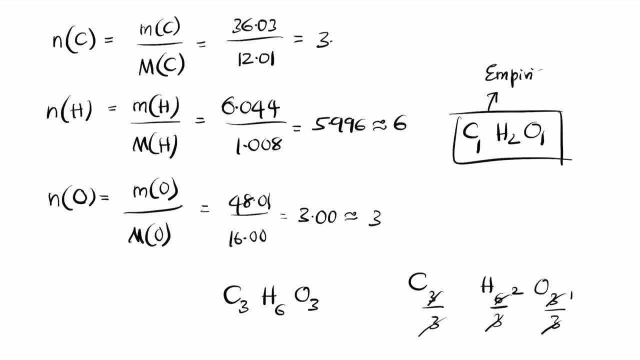 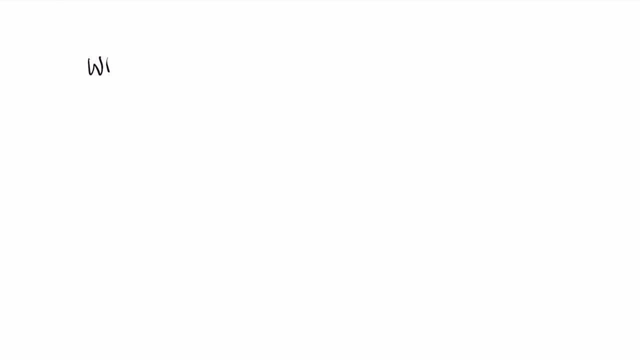 So this here is the empirical formula. So to find the molecular formula now you need the whole number multiple. So the whole number multiple is the molar mass by the empirical formula mass. So we want to find the empirical formula mass. 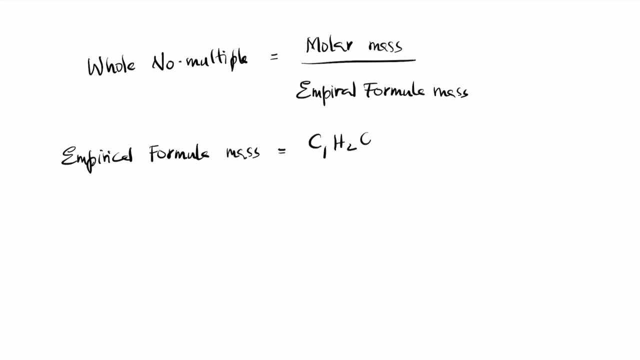 So empirical formula is C1H2O1.. So that is 1 times C1H2O1.. So that is 1 times C1H2O1.. So that is 1 times C1H2O2 plus 14 times 15.LIEU plus 5 times C1H2O3 plus 14 times. 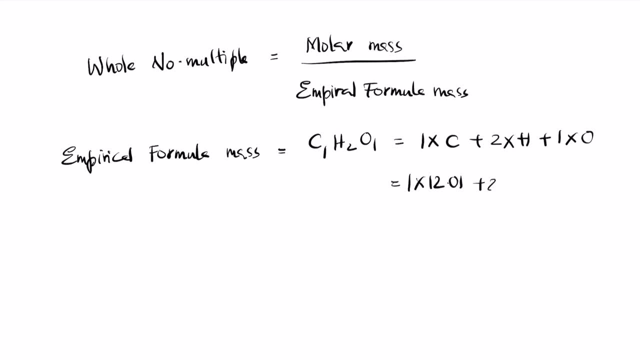 Cy3C2O3 plus 14 times C1H2O3 plus 5 times 23.. Ma that has been a Derby or context. so there is a T Am T Ira, which is hetero equation. 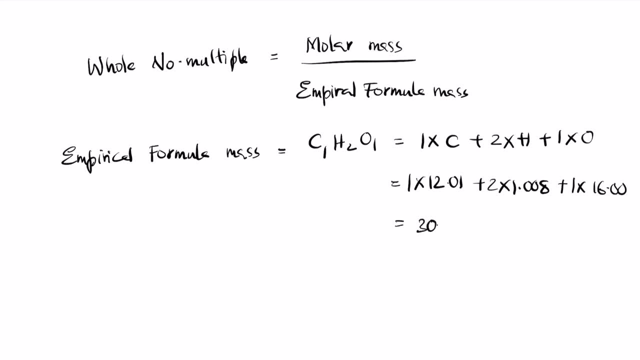 So prototips wouldn't work. Let's talk about the Z1s. So that is topological languages. So that gives you a value of 30.03 grams. So molar mass is 90.08 over 30.03.. So 90.08 divided by 30.03 gives you 2.999.. So which is nearly equal to 3.. 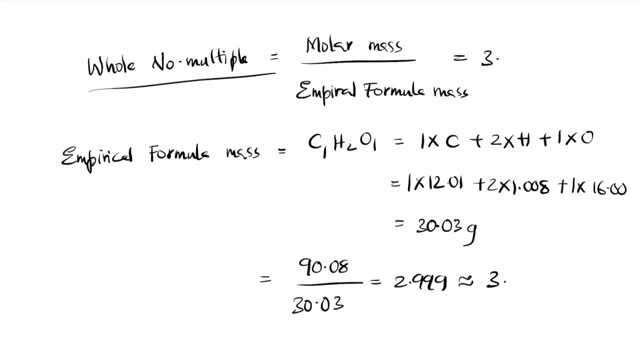 So the whole number multiple is 3.. So to find the molecular formula, so multiply the whole number multiple with each of each the molecular formula, So CH2O, so times the whole number multiple is 3.. So that becomes CH3H6O3.. 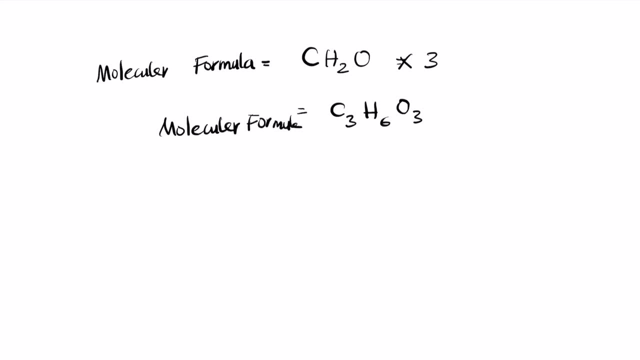 So this is the molecular formula, C3H6O3, and the empirical formula is C1H2O1.. So this is how you can solve the problem and find your final answers. So let's try another example. So this time you try this example. 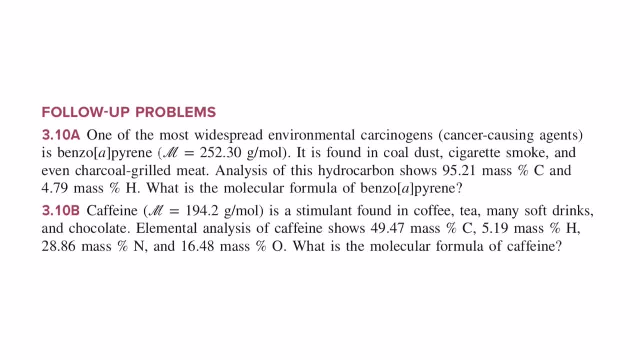 So try these two problems. So here you can see that you have two problems. So here you can see that you have two problems. You have molar mass given, so molar mass is given and they've given us the mass percentage. so similar to the last problem. 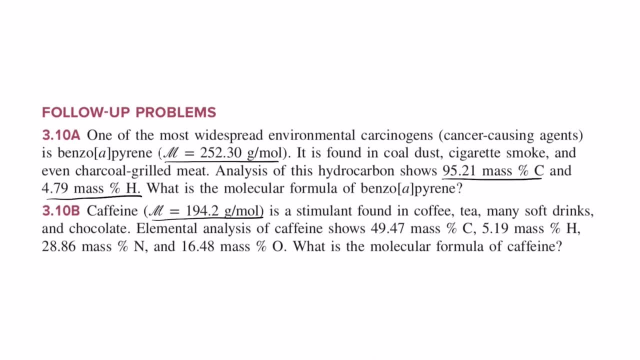 Next in caffeine also. you have the second problem. also you have the molar mass and you have this time four elements. So mass percentages are given. so try to calculate from the. so try these two problems. So pause the video right here and try to calculate for these two problems. 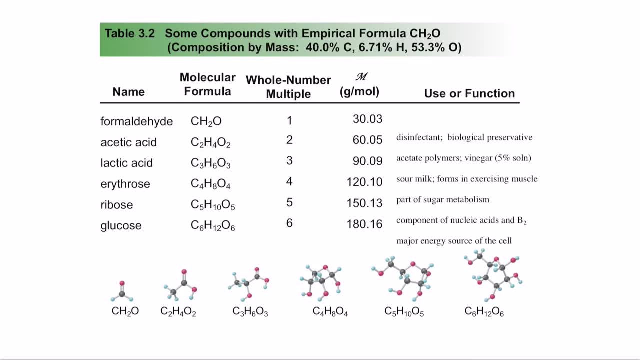 So the reason we don't use empirical formula more often is because there's a significant difference. often is because compounds can have the same empirical formula but have different number of each of these. in the molecular formula, for example, all of these compounds have the same empirical formula, ch2o, but every one of them has a different purpose and a different use, and also 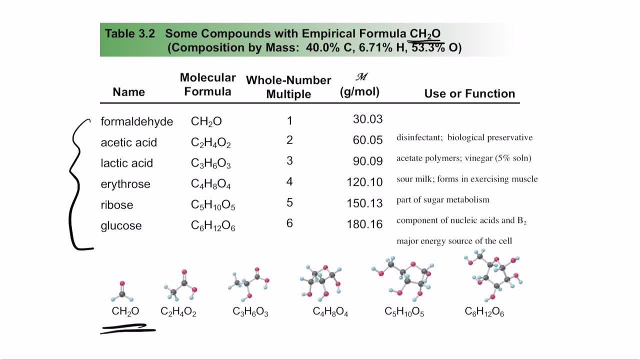 has a different structure as well, so which means that empirical formulas are not that useful in representing the structure, but they are useful in representing the actual mass of each individual element. notice that all of these are multiples of each other, so they can be used as well, but the 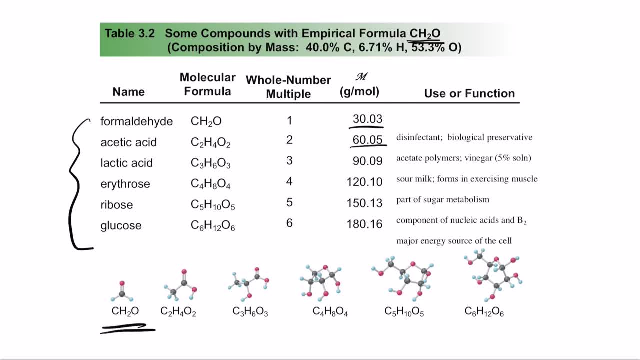 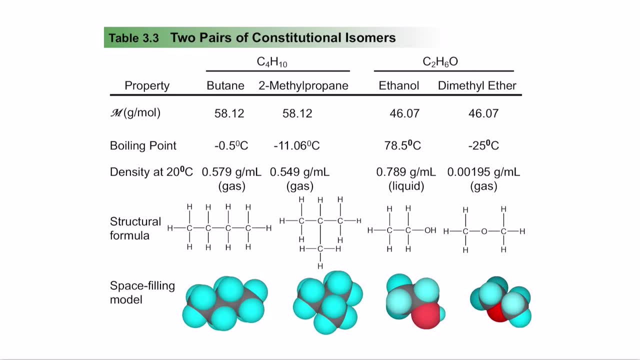 thing is they are not generally used as an empirical. formulas themselves cannot be used to represent the structures. the same thing happens when you have two molecular formulas with the same structure but they can have the same properties. so for example, even two molecular formulas, even if you have a single molecular formula, two molecules with the same molecular formula can. 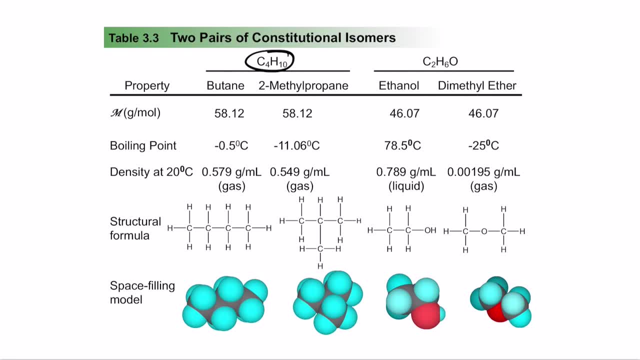 have two different properties as well. so molecules with different connectivity and the same molecular formula are called constitutional isomers. so remember the name. you're going to hear it again and again in organic chemistry. so whenever you see the term constitutional isomers, these are molecules with the same. 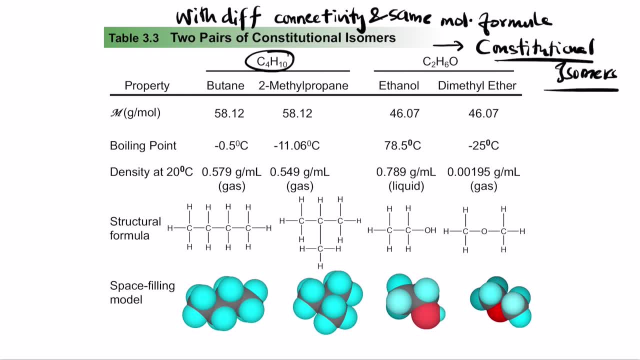 molecular formula. but the molecules are arranged. the atoms in themselves are arranged in a different order. for example, if you look at the carbons, notice the carbon arrangement is much more different in both the molecules. in the same way, in these two elements as well, the attachment of oxygen here is different from a different in each of these. 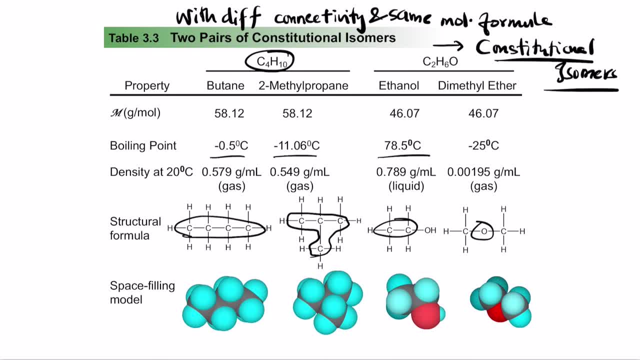 elements provided. that's why, you see, there is a difference in their boiling points, their, their densities, their structural formula and also their space filling models, even though their molecular molar mass stays the same. so this is why structures cannot be represented just by either the molecular formula or the molecular formula. so these are the two elements that are different.